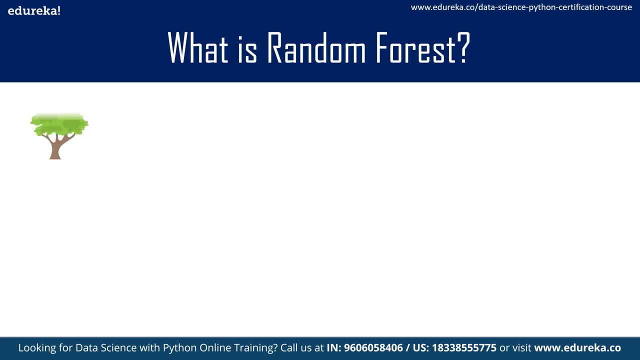 me make things very simple for you by taking an example. Now suppose we have got three in the pending decision trees. Here we are just taking three decision trees and I've got an unknown fruit and I want that these trees would give me a result of what exactly this fruit is. So I pass this fruit. 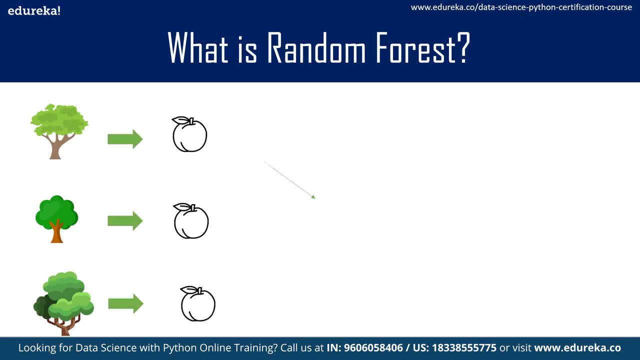 to the first decision tree, the second decision tree and the third decision tree. Now, a random forest is nothing but a combination of these decision trees, So the results are being fed into the random forest algorithm. So what it sees is that: okay, the first decision tree classifies it. 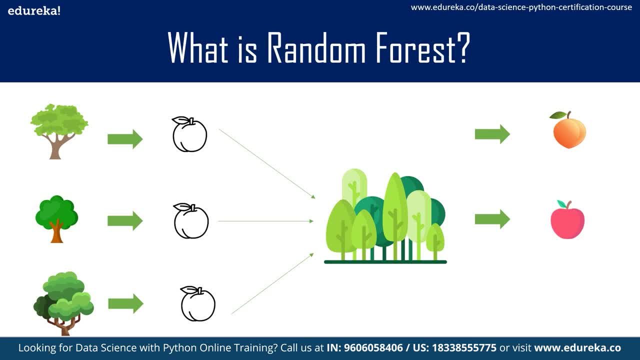 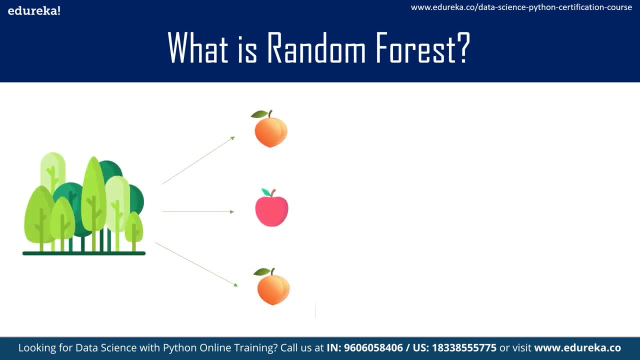 as peach. The second decision tree says that it is an apple and the third one says that it is a peach, So random forest classifier says that. okay, I've got the result as two peach and one for an apple. So I would say that the unknown fruit is an peach. All right, so this is based on the majority voting of: 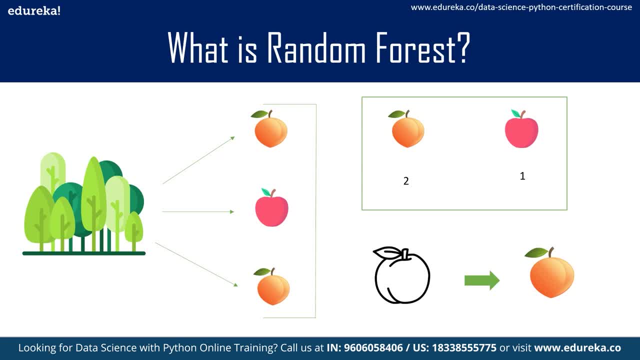 the decision trees, and that is how a random forest classifier comes to a decision of predicting the unknown value. Okay, so this was a classification problem, So it took the majority vote. Now suppose if it was a regression problem it would have taken mean of it. Okay, so now let's move on further to understanding what is a decision tree. But before 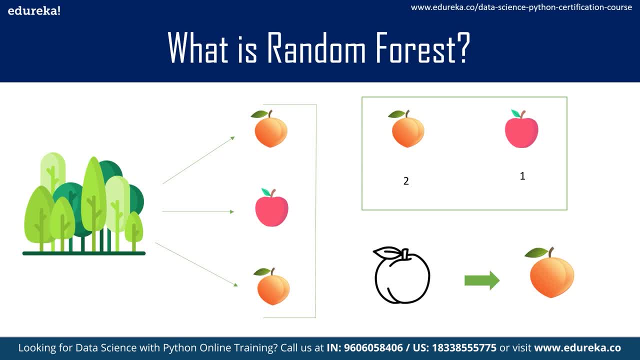 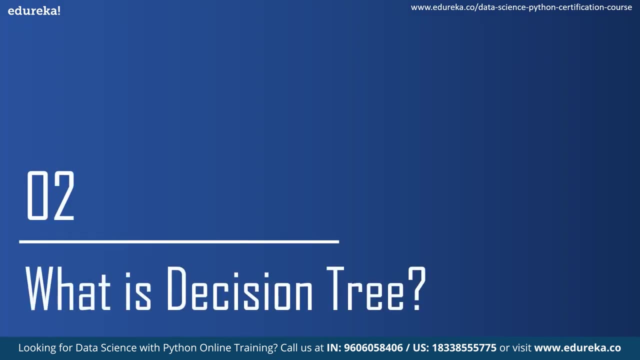 that we should understand that random forest. the building blocks are decision trees, and that's why studying decision tree becomes important, because if we understand one decision tree, we can apply the same concept to random forest. Okay, so let us understand what is a decision tree? So decision. 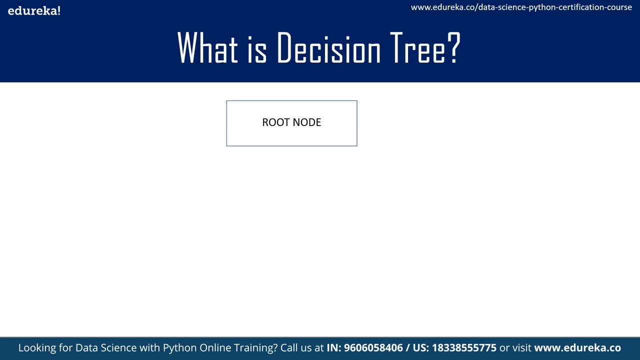 tree is basically three nodes that are important. The first one is the root node. The root node, as the name suggests, here the data set, the entire data set, is fed at the root node. And then there are decision nodes where decisions are being taken and splitting is performed, And then we've got the leaf. 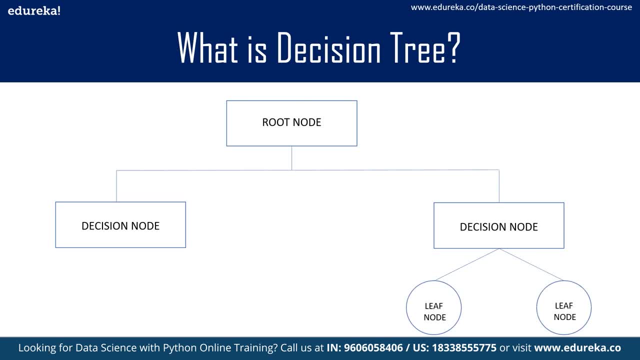 node and these leaf nodes are the ending point of the tree, where no further division takes place, And we can say that the predictions are made at the leaf nodes. Okay now, another thing to note here is that Decision nodes provide links to the leaf nodes and decision tree breaks the data set into smaller 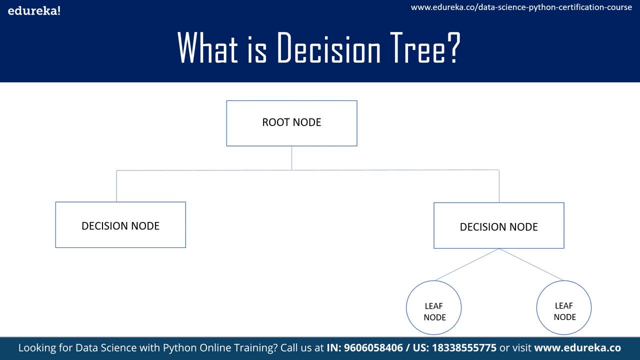 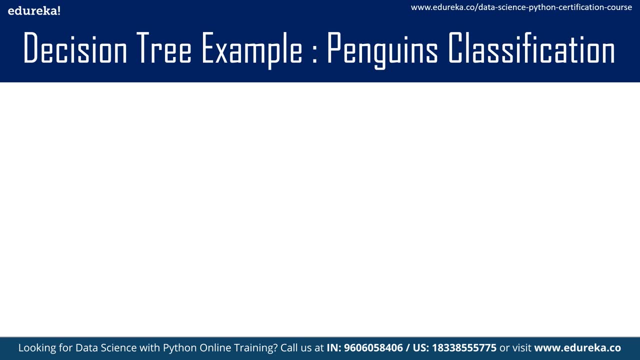 subsets, Splitting is done at nodes and at the end of the tree, the final point, the decision or the prediction, is made. Now let's construct a decision tree and take an example of the penguins classification. So let me just walk you through. what is this penguin classification problem? So 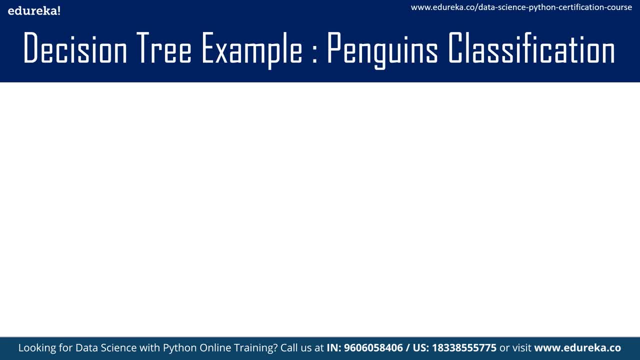 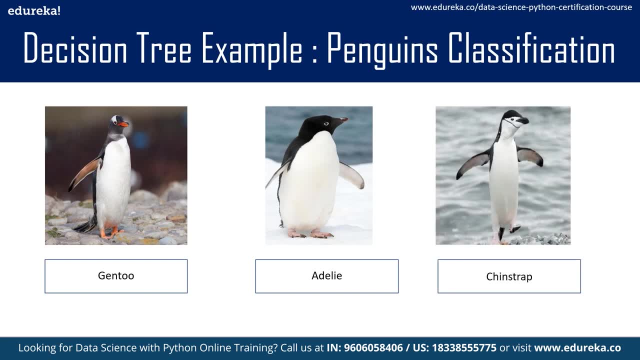 we've got some three species of penguin. Let us get familiar with these penguin species. This is kentos, This is elderly and this is chinstrap species. So these are the penguin species of Antarctica and they are found on different islands. So we have to classify these penguin species correctly. So we're using 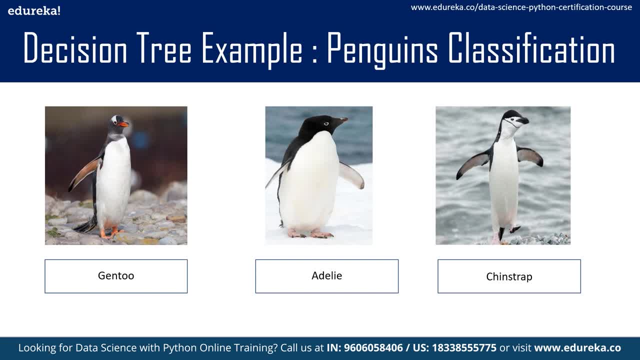 random forest here, But for convenience sake, let us just walk with decision tree right now and we'll see how a decision tree really classifies these species. So that's really interesting And let's move on forward and understand some parts of this penguin, because we'll be working with this data set. 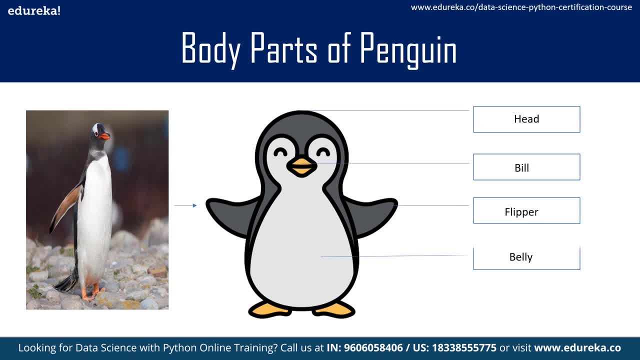 Okay, So this is a penguin and this The head, bill, thipper, belly and claws- the different body parts of the penguin. So we are majorly concerned with the bill and flipper and the body mass of the penguin because that data set contains majorly of these features. So make sure that you understand. 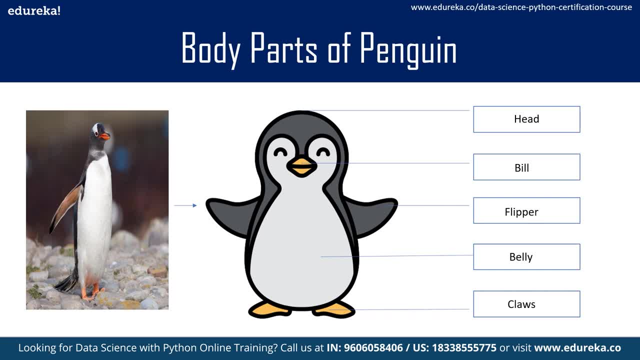 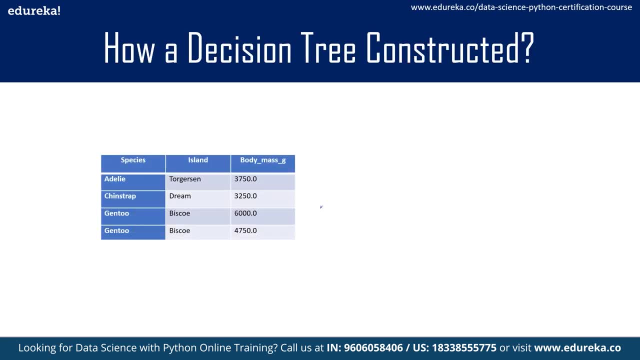 the flippers and also the fill of the penguin. Okay, so now moving on forward and let us now construct a decision tree. So let's see how our decision tree is constructed. So I have taken a subset of the penguin set. 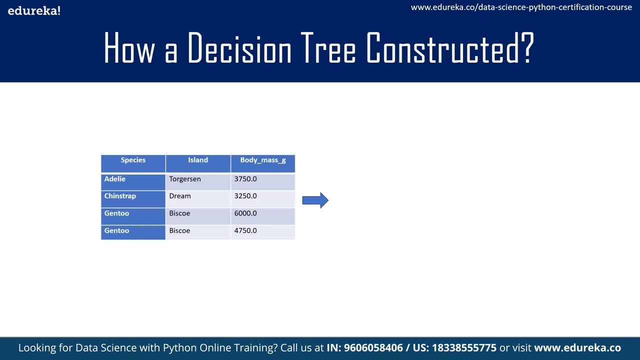 data and here we see only two columns, that is, island and body mass and of course, the species of the penguin. that is the outcome or the target variable that we have in this subset. so now we construct a decision tree here and we take body mass as the first feature and the splitting is done based on one. 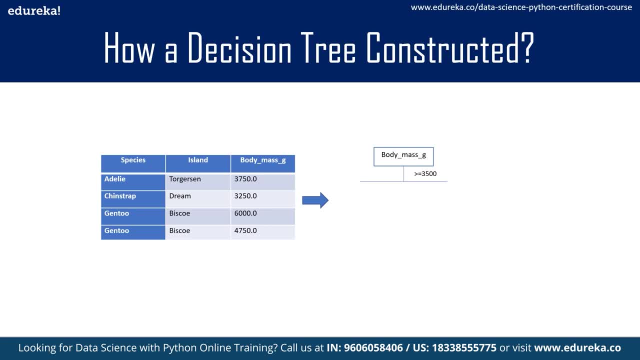 condition that if the body mass is greater than equal to 3500. and if it is YES, then based on island- another feature- we will classify, or get the leaf node, as either tigressan or Bisco Island. so if the island is either tigressan, then the specie would be ediments, And if the island is Bisco, then the 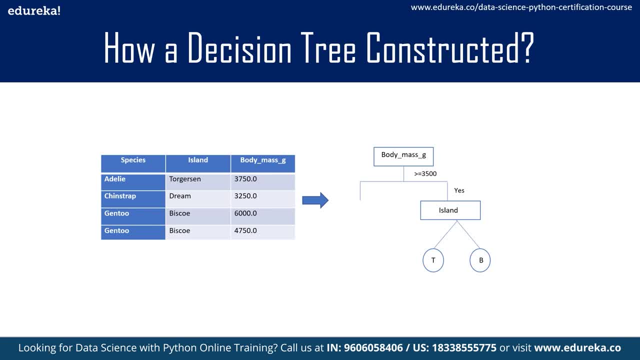 specie would be Ghentos. So after tigressan and Bisco, no further division takes place, because we are getting the predictions and these leaf nodes, whereas if the body mass is less than equal to 3500- and it says that, yes, the 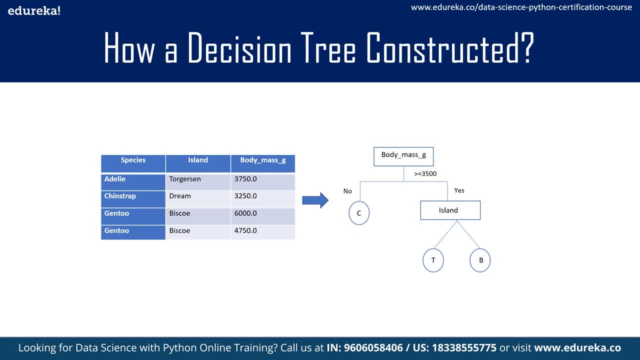 body mass is less than 3500, so we get the species as chin strip and so no further decision had to be made at this node and that's why it was been ended here. So this was a very simple, basic example of a decision tree, and suppose if we had got a huge data set this decision tree would have gone into. 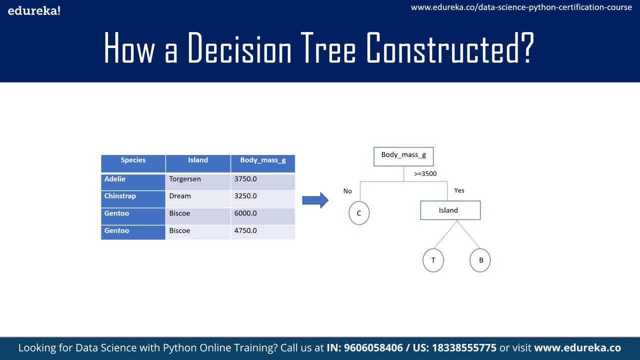 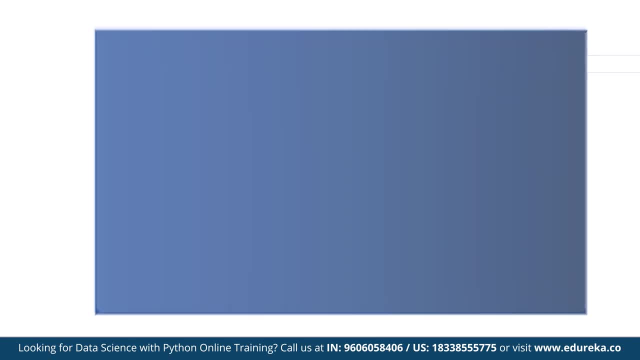 a huge depth, and the depth of the decision tree would have led to overfitting of the data. So that is one of the drawback of decision trees that random forest overcomes. So now let's move on forward and understand the important terms in random forest, and this will also help us consolidate. 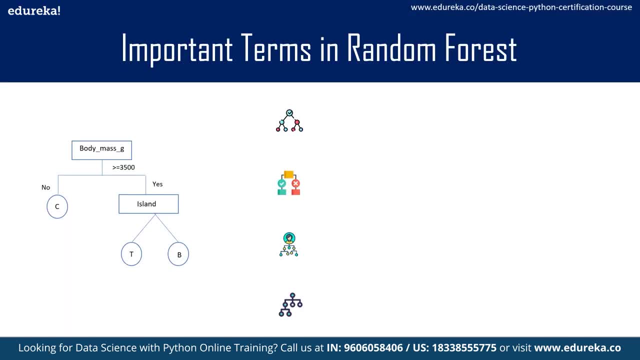 whatever we have learned so far. So we've taken the same small decision tree of the previous example and let's understand. these are also the important terms which will be relevant to random forest also. So the first is the root node. Now, here, what happens is that the entire training data has 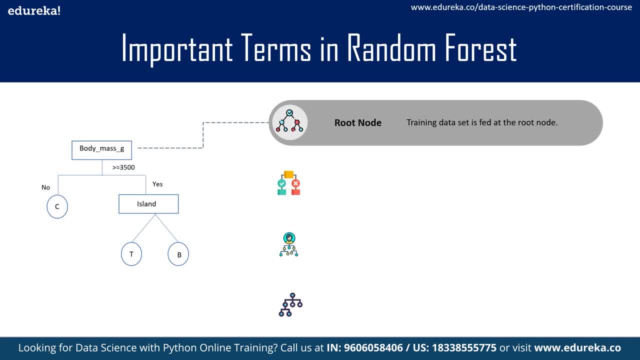 been fed to the root node. and then we've got here that each node will ask either true or false question with respect to one of the feature and then, in response to that question, it will partition the data set into different subsets. That's what it is. 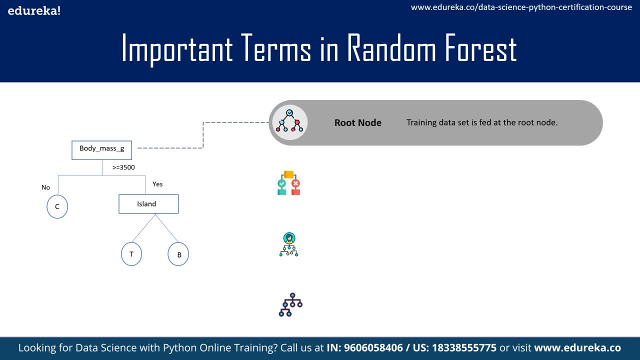 it is doing here, based on the condition that if the mass- body mass- is greater than equal to 3500, it asks a question, either yes or no, and based on that again for the partition is done, and if not, then it just classifies the species and then again what happens is that the splitting. now this is very 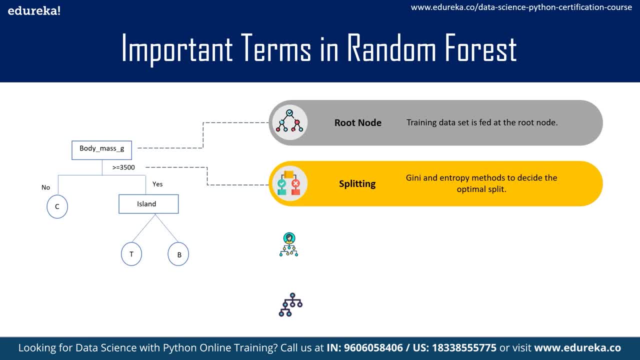 important here. The splitting takes place either with the help of a genie or entropy methods, and these helps to decide the optimal split, and we will be discussing about splitting methods very soon, right, Okay. and then we've got the decision nodes, which provide the link to the leaf nodes, and these are really important. 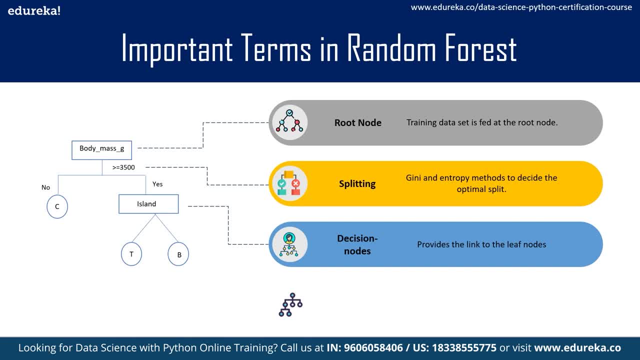 because then only the leaf nodes will tell us what actually the real predictions or to which class does the species belong. So now coming to the leaf node, and these are the end points where no further division will take place and we will obtain our predictions. Okay, so now coming up. 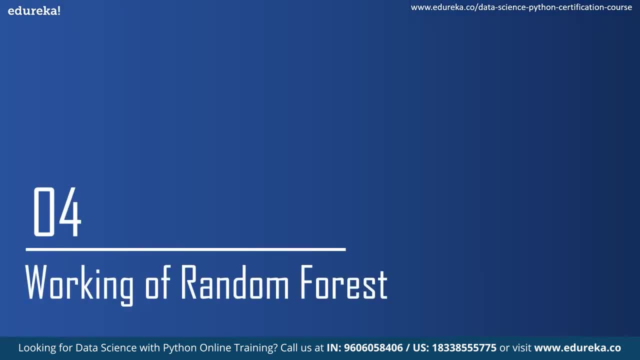 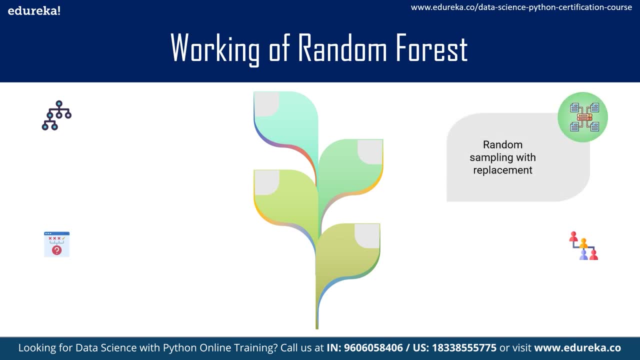 to another important thing here is working of random forest. So now for working of random forest, we will have to understand a few important concepts like random sampling with replacement, feature selection and also the ensemble technique which is used in random forest, and that is bootstrap aggregation, which is also known as bagging. So we will understand this with the help of an example. 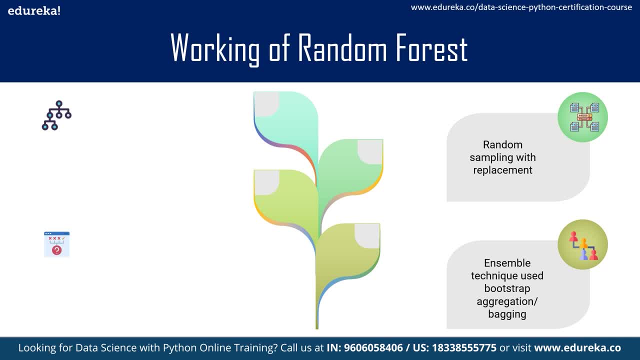 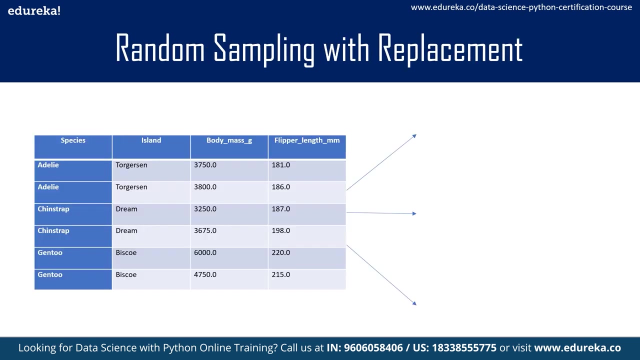 Which will be very simple. and then we will go on understanding how feature selection is done in both the classification and the regression problem. actually, how random forest select features for the construction of decision trees? Well, in random forest the best split is chosen based on genie, impurity or information gain methods. So this also we will understand. Now let us first understand. 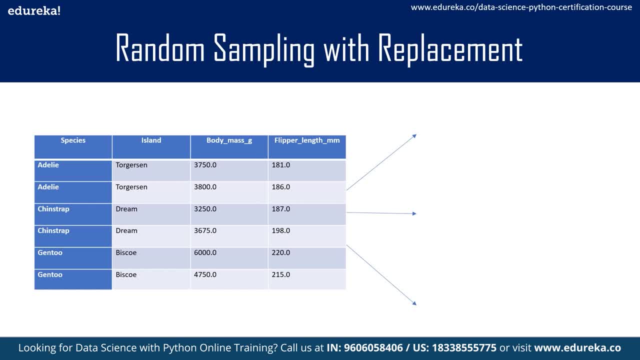 random sampling with replacement. Now, what happens here is that we have got a small subset of the same tree. Now, what happens here is that we have got a small subset of the same tree. So we will understand how hombresick name, Penguin data set, Wherein we have got some 6 rows and four features. 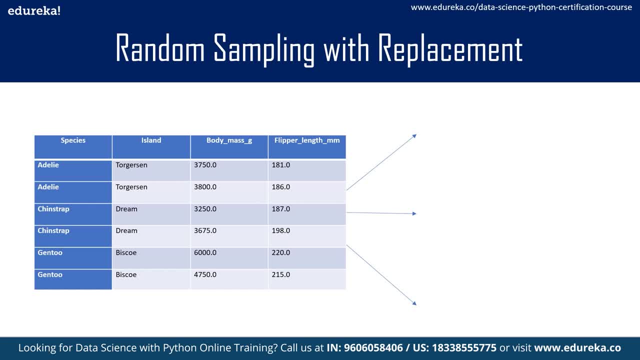 that means 4 columns And the arrows that you can see is that now we will be creating three subsets from this small subset, Right, and these three subsets will become our decision trees, and then we'll be constructing decision trees from these subsets. So let us create our first. 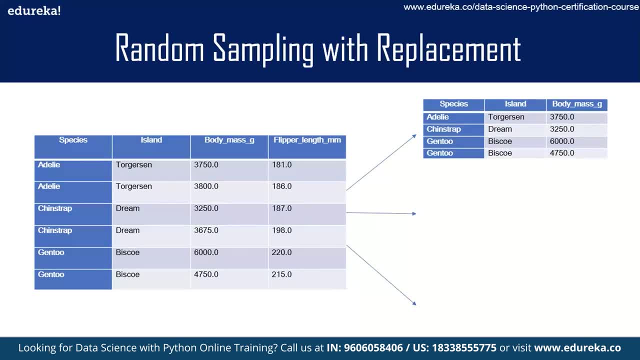 subset and you can see here that this subset is randomly being created. and for convenience sake, let me just also show you the different subsets here here. okay, so now for better understanding. let us understand this: that in the first subset, if we focus, we've got certain random rows here and 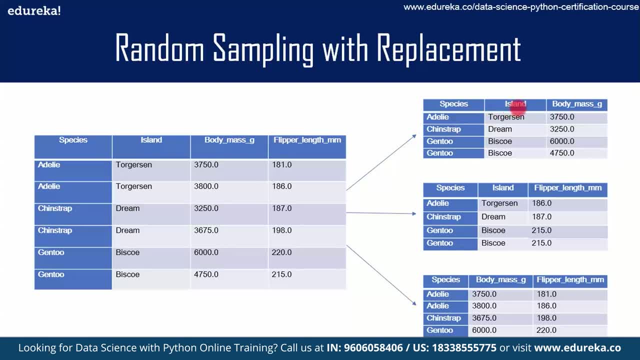 we've got certain feature, but we do not know how this feature has been selected. we got island and we got body mass, but in the second subset we got island and flipper length, and in the third subset we got body mass and flipper length. right now, let's look at the rows now. when I am talking about these features, I 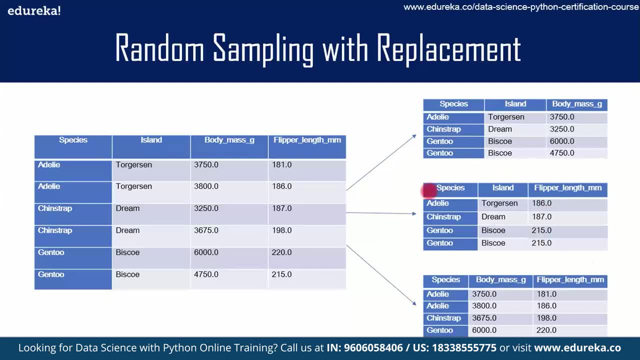 will say this is feature selection and remember this term. now coming to the second concept, that is, random sampling. now, random sampling is nothing but selecting randomly from your subset. so I'm selecting randomly certain rows from my subset and creating for the subset okay, so what is replacement here? 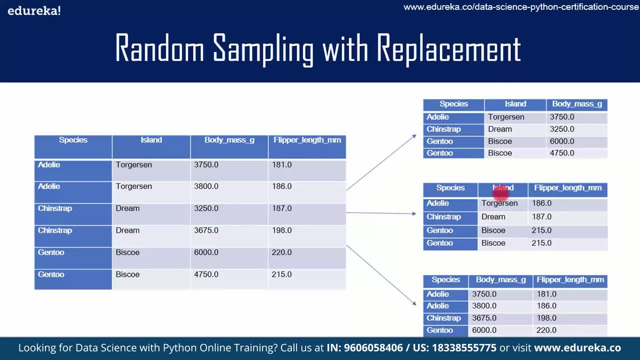 replacement is can be seen here and can be understood with this second subset. we see here that the Gentile species, this row, is being repeated again as: and this is replacement. that means that when we are working with repeated rows and this row can be repeated again in the second or the third subset, then this 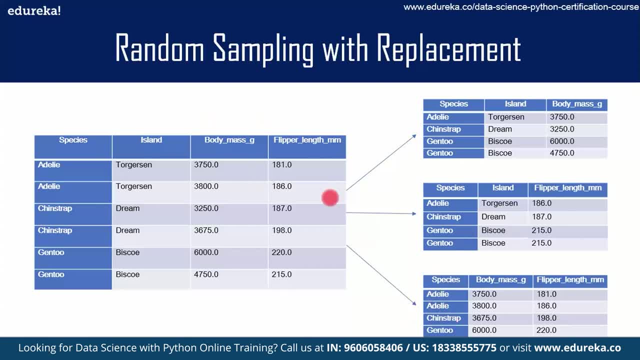 is random sampling with replacement. that means my random forest can use a row multiple times in multiple decision trees. right, so this is the basic concept of random sampling with replacement and feature selection in random forest. another important term which I would like to bring into the notice is that when we are working with these type of small subsets, these are: 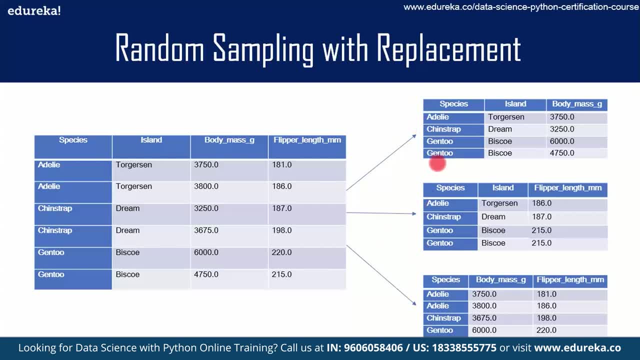 also known as a bootstrap data sets, and when we aggregate the results of all these data set, it becomes bootstrap aggregation. so just filling in the gaps so that later on the concepts become more clear. so now let's move on to drawing decision trees of these subsets. okay, so let's draw the decision tree of. 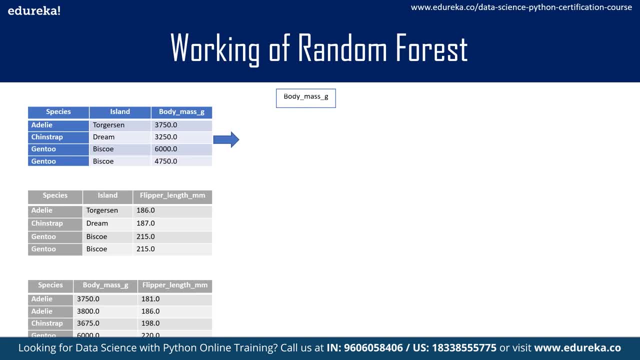 the first subset. again, we are taking body mass as the first root node and then, based on a decision like if the mass is greater than equal to 3500, then take a decision either yes or no. if it is no, then the specie is chinstrap, and if it is yes, then again you partition based on island. 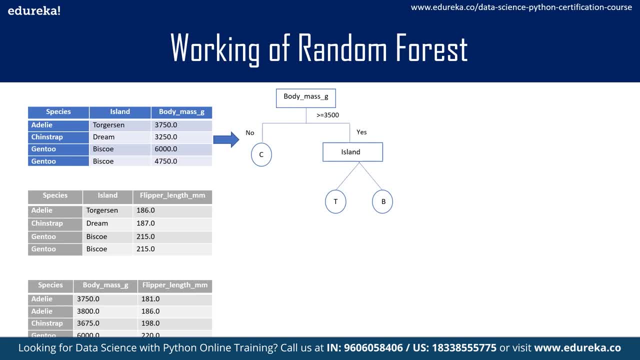 and if it is tougresen, then it is adly, and if it is visco, then it is Gentile species. okay, so this is how we will construct two more decision trees of the remaining subsets, so the second subset. let us just again create decision tree. 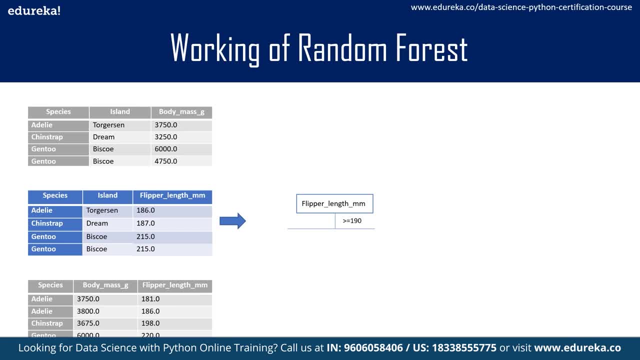 and here now we are taking flipper length, and then based on a condition, that if the flipper length is greater than equal to 190, then make a split. if it is yes, then the specie become Gentile, and if it is no, that means again make a. 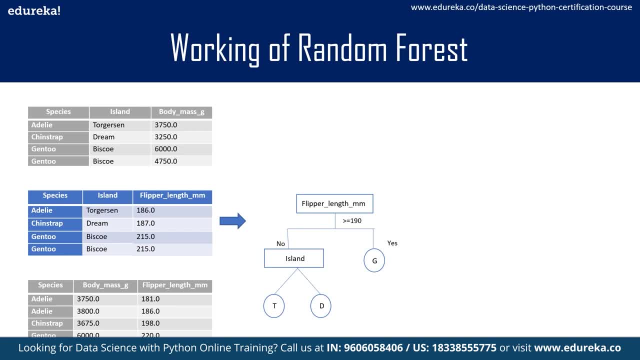 decision based on island, and if it is tougresen, then it is adly, and if the island is dream island, then it is a chinstrap specie. so this is how the decision tree of the second subset has been created and this is how it will take. 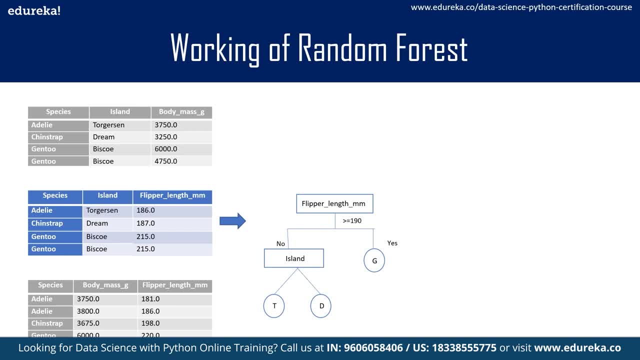 decisions right, based on the tree length, depth and also the features it is selecting. okay, so now let's create the third decision tree of the third subset and we get a decision tree something like this where, in body mass, if it is greater than 4000- and if it is yes, then clearly it is a Gentile species and if it. 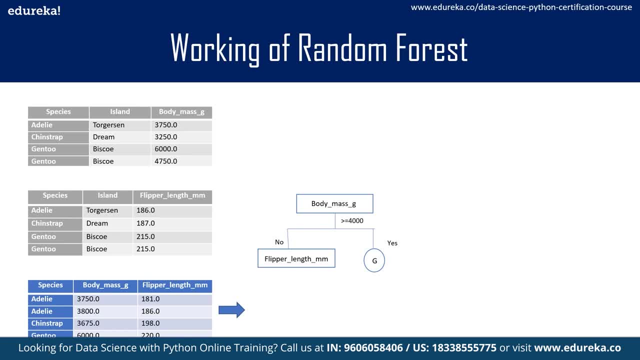 is no, then again make a partition with the respect to flipper length- another feature here- and then if it is again greater than equal to 190, then the specie would be adly, else it would be chinstrap. so this is our decision. tree 3 will make a decision. now let's just keep these decision trees. 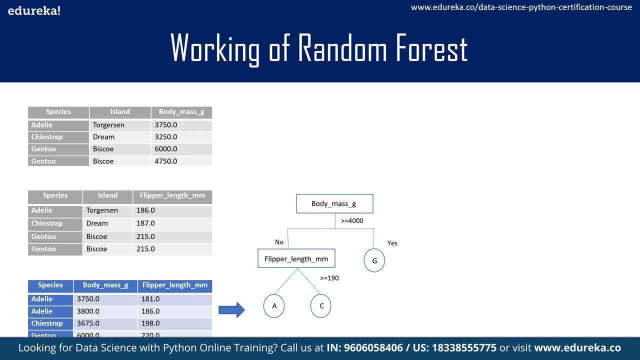 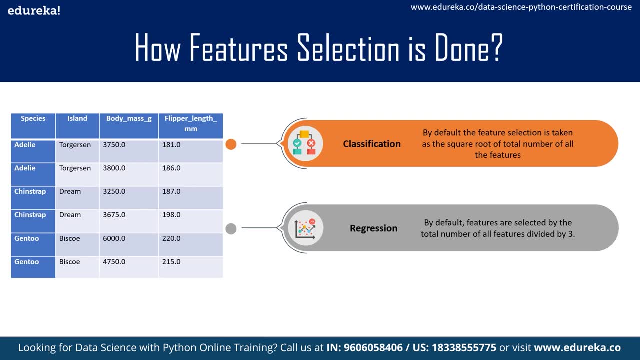 with us. okay, and we will make sense of these trees just in a while. okay, but before that, let us understand how feature selection is done in a random forest. how am i selecting the columns? so for classification, by default the feature selection is taken as the square root of total number of all the features. 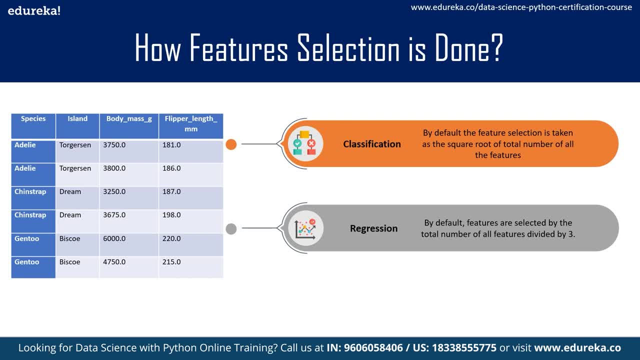 now suppose I got here for features, So it is a classification problem. I will take the square root of these four features, which becomes 2, so decision tree would be constructed based on two features each. is suppose I had 16 features, then it would be square root of 16, that would be 4. 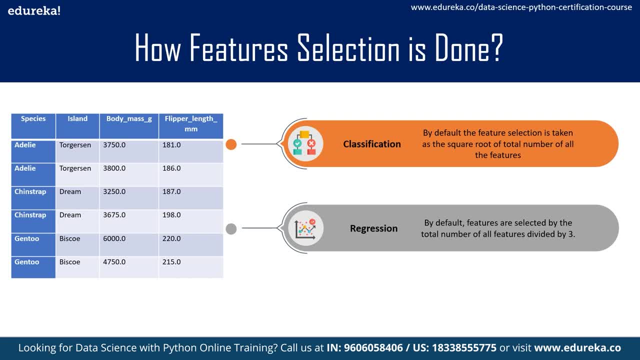 so 4 features would be taken in each decision tree. All right, and suppose if this would have been a regression problem, then, by default, what would happen? the features would be selected by taking the total number of features and dividing them by 3.. Okay, so this is how, by 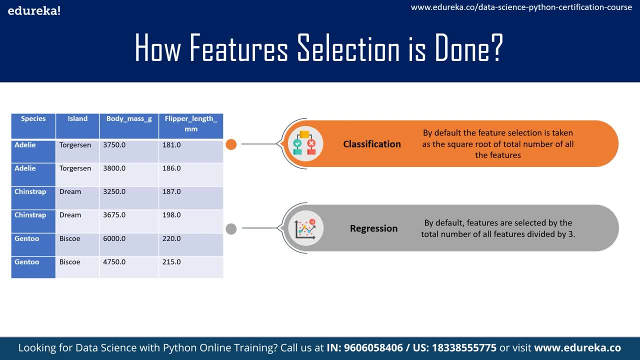 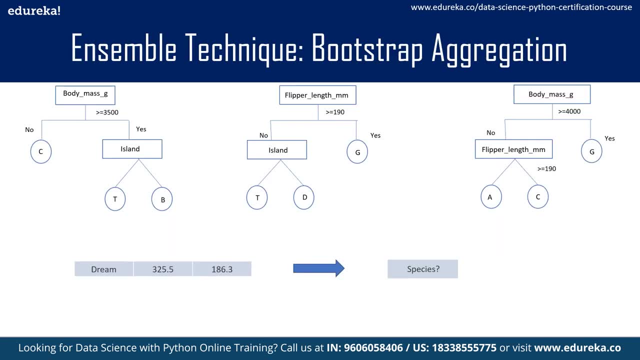 default, the feature selection is being done by a random forest. Okay, Now let us move on forward to consolidating our learning. So now we are coming to ensemble techniques. that is also known as bootstrap aggregation. random forest uses ensemble techniques. and what is assembling? it just means that you are aggregating the result of the decision. 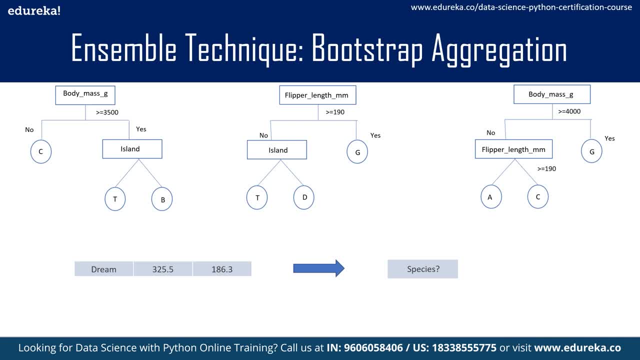 trees and taking the majority vote in case of classes, Specification and the mean in case of regression problems, and giving the output Okay. So now we have again plotted all our decision trees here and below we can see that there's an unknown data and I want to predict the species of these data. So what will happen is that. 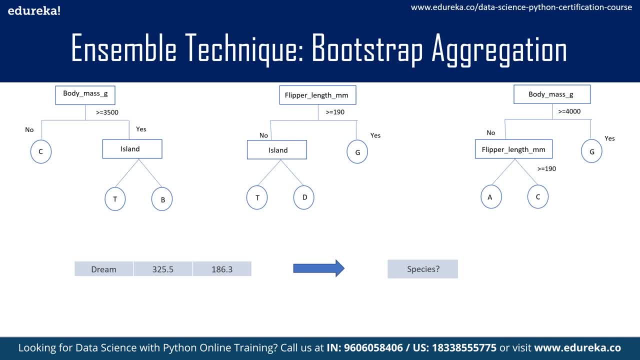 again, let us just feed this problem to each of the decision tree and let's see what each decision tree makes the prediction. So I just feed this unknown data to decision tree one and it says that, Okay, the specie seems to be chinstrap. Okay. and then decision tree two says that, based 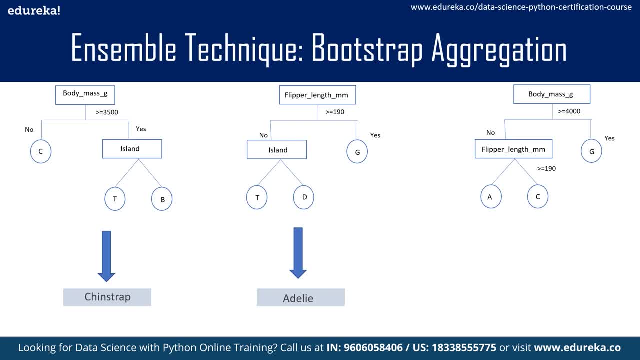 on the data, it has been found that the specie is Adelie. and then decision tree three says that: no, I with my decision tree, this specie is chinstrap. Okay, Now all these data is being fed to random forest classifier and it says that: okay for chinstrap, I've got two. 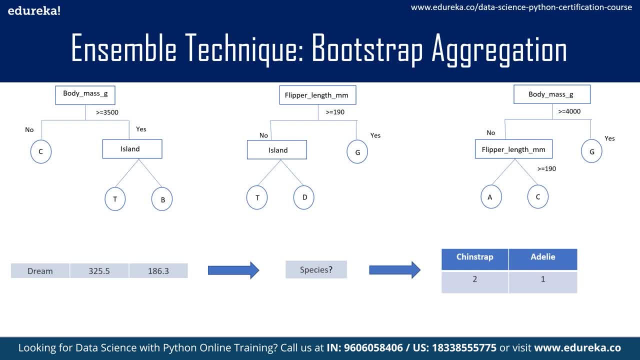 votes. for Adelie, It's got one vote, So the new specie would be chinstrap. Okay, so now this is how the bootstrap aggregation is done: based on the majority voting and the decisions taken by different decision trees, They have been combined together, aggregated and we get 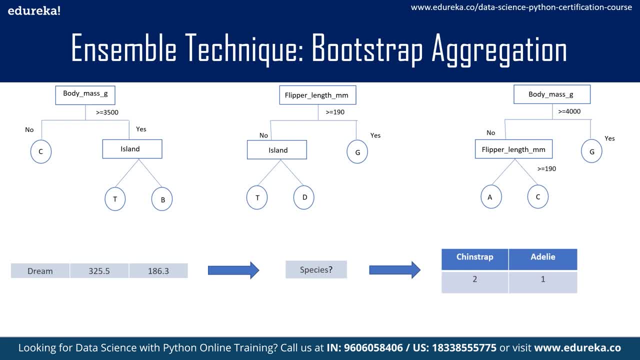 an ensembled result in the random forest. Okay, so this was very simple concept of ensemble techniques which has been used in random forest. Okay, so now let's move on forward to splitting methods. So what are the splitting methods that we use in random forest? 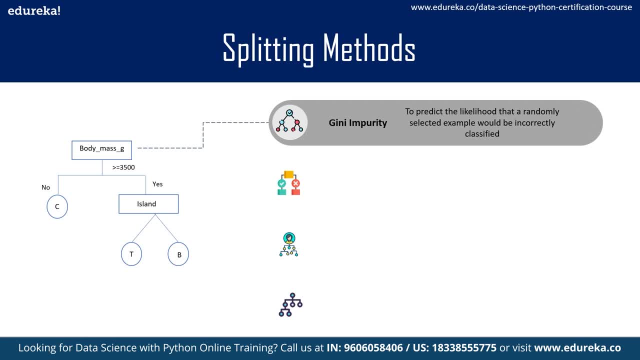 So splitting methods are many, like Gini impurity, information gain or chi-square. So let's discuss about Gini impurity. So Gini impurity is nothing, but it is used to predict the likelihood that a randomly selected example would be incorrectly classified by a specific node, and it is called 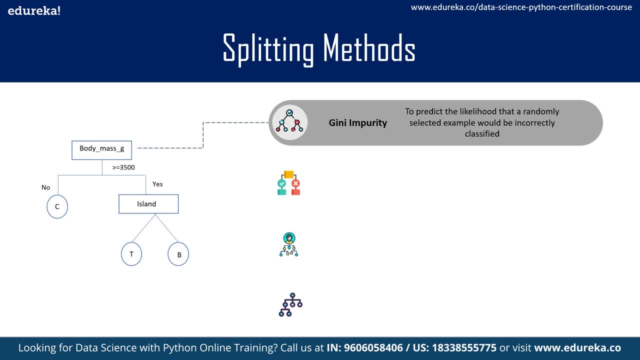 impurity metric because it shows how the model differs from a pure division right. And another interesting fact about Gini impurity is that the impurity ranges from 0 to 1, with 0 indicating all of the elements belong to a single class and one indicates that only one class exists. 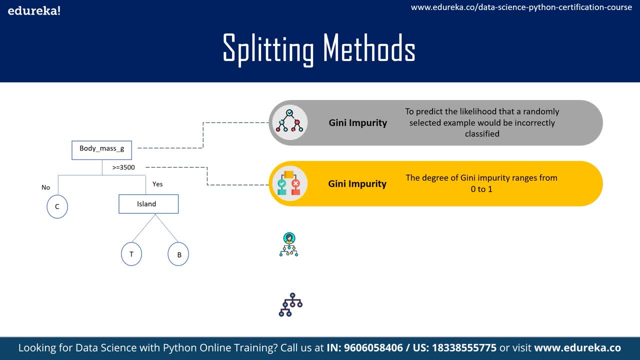 Now value which is like 0.5. This indicates that the elements, they are uniformly distributed across some classes. right Now, moving on forward to information gain. Now, this is another splitting method which random forests can use, and information gain utilizes entropy. So entropy is nothing, but it is a measure of uncertainty. So information gain, let's. 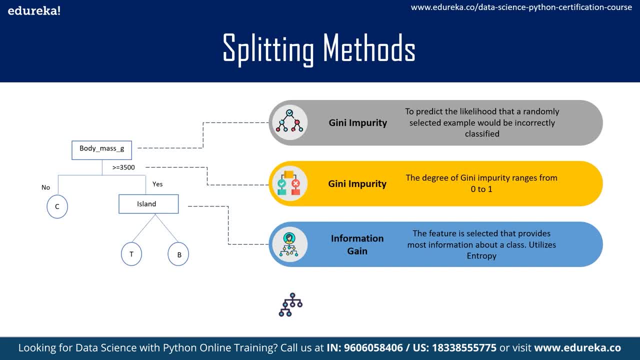 talk about that first. So the features: they are selected. that provides most of the information about a class right And this utilizes the entropy concept. So let's see what is entropy? This is a measure of randomness or uncertainty in the data right. So we will understand this entropy. 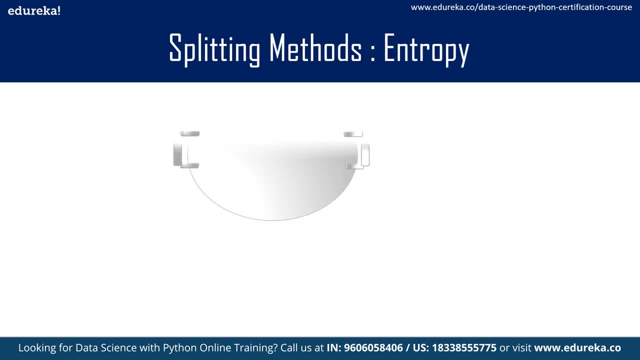 with the help of a small example. So don't worry about it. So let's understand this entropy. Now suppose there's a fruit tray with four different fruits, right, And what do you feel about the entropy here? That means a randomness of the data. Is it really easy to classify these fruits into? 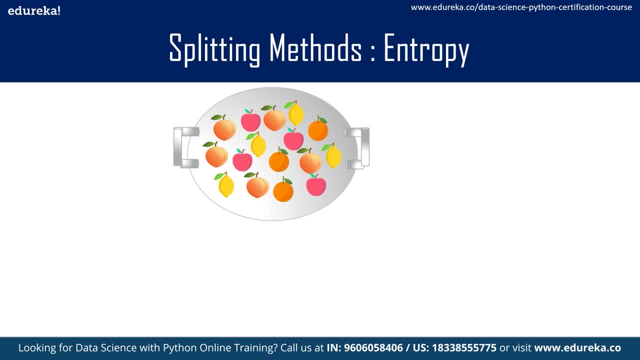 the respective class. So this becomes really uncertain and the data looks messy here. But what if we just split here these into two trays, where in the first tray would have peaches and oranges and in the second tray will have apples and lemons? So now this becomes a little. 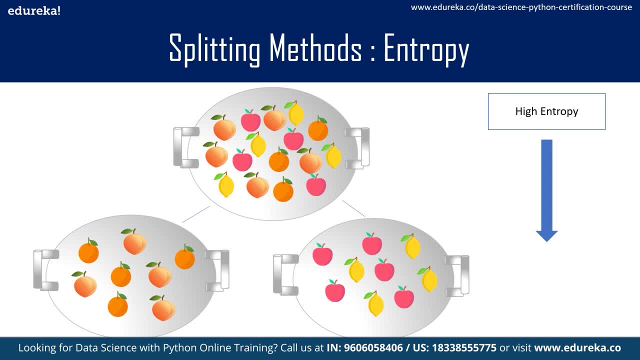 more certain. we get low randomness here and this is called as low entropy. So when we move down from tree- That means from root node to the leaf nodes- the entropy reduces and we can also calculate information gain from this entropy. That is the difference in entropy before and after. 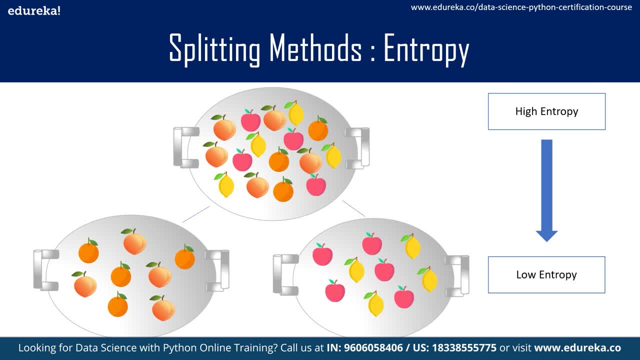 the split that is known as information gain. Okay, so once we move down the tree and start reducing the randomness from the data, the entropy becomes lower, and that is what we want in our data. If there's low entropy, that means we are likely that the predictions 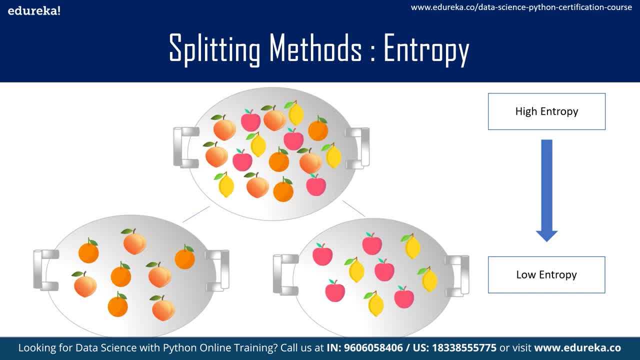 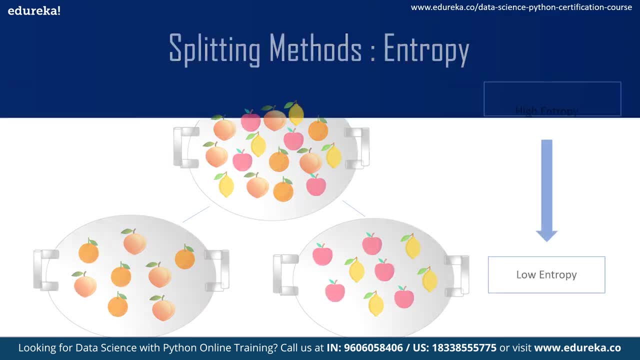 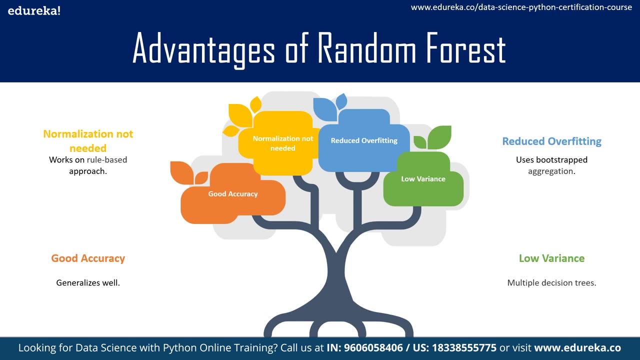 would be more accurate And we can make predictions very easily, as compared to very messy data which has high entropy. Okay, so that was about entropy. So now let's move on to understanding the advantages of random forest, and we see here various advantages, So let's focus on firstly: 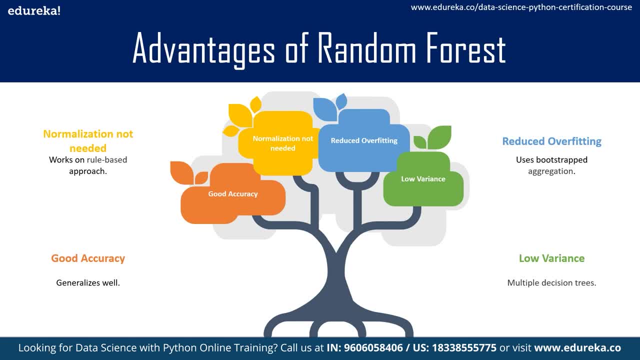 low variance Now, since random forest overcomes the limitations of decision tree and it also has the advantage of low variance because it combines the result of multiple decision trees. So the decision tree is being trained on limited data set that we have seen earlier also. So 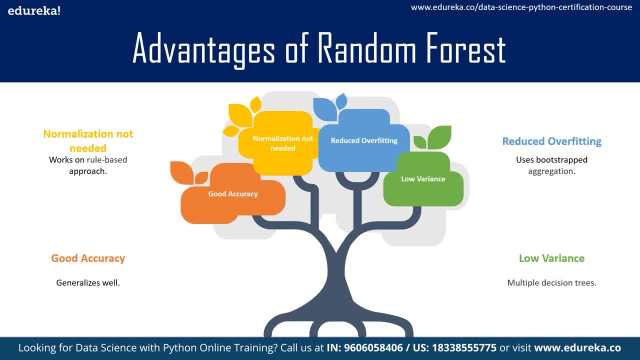 each tree was making its own subset of data and training the data on that limited length of the tree. So there's less depth, there's less overfitting and low variance of the data. So, coming to the next point, that is, reduced overfitting Again, since we were working with multiple. 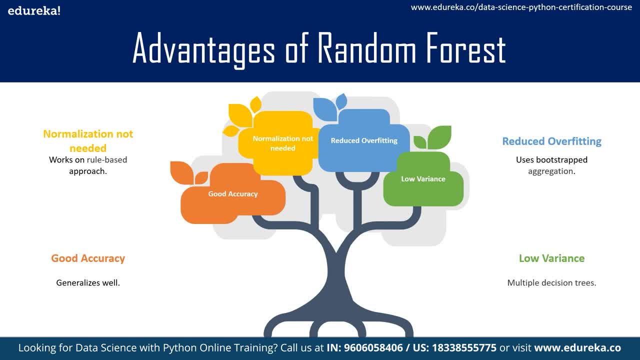 decision trees, hence reduced depth of the tree. So we get reduced overfitting. That means the model is fitted well and it does not try to Learn even the noises Right. So we use the bootstrap, aggregation or bagging here in random. 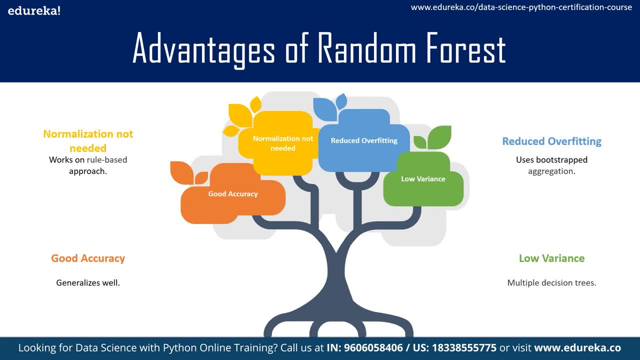 forest, and that is why we also get reduced overfitting in random forest. And this is one of the reasons that. why is it so popular? because you don't have to worry about overfitting of the data Right, All right. Now moving on forward to the another advantage is that the normalization 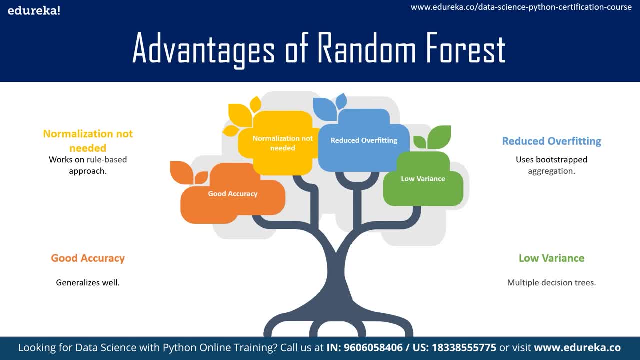 is not required in random forest because it works on rule based approach Right, And another advantage is that it gives really good accuracy, which we will also see in our hands-on. It really gives a very nice predictions, either precision or recall, and generalizes well on unseen data as compared to 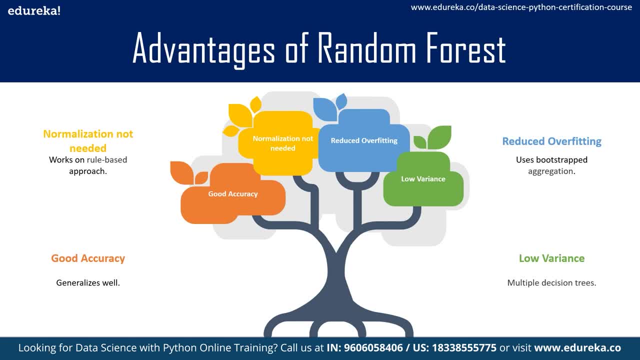 other classifiers or machine learning classifiers which are present, like Naive Bayes or SVM or KNN, Random forest really outperforms other classifiers right. So let's move on to understanding a few more advantages of random forest is that it is suitable for both classification and regression. 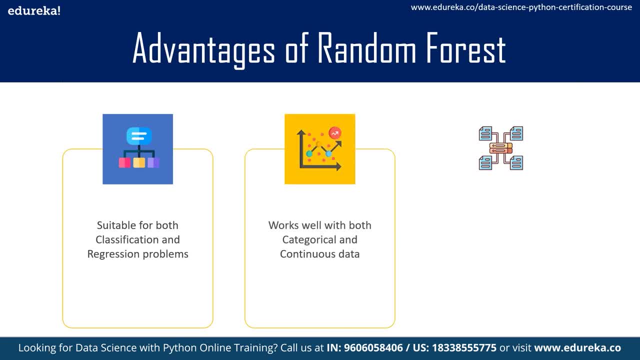 problems, And also it works well with both categorical and continuous data, So you can use it well with any of the data sets right, And it performs well on large data sets right, So it solves most of the problem. That's why random forest is largely been used in machine learning. 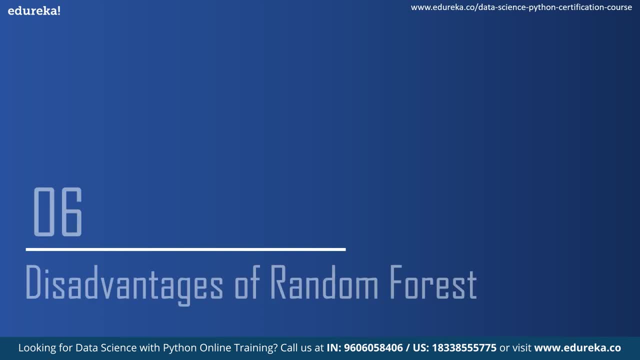 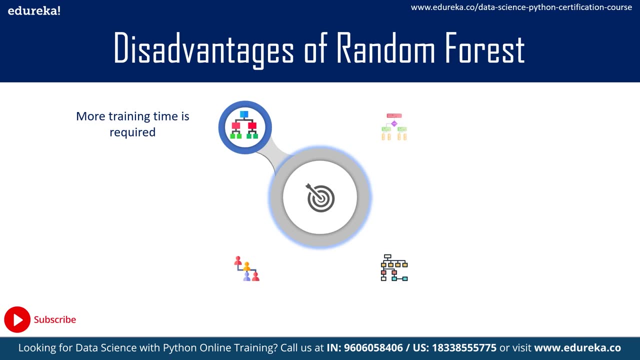 problems. Now moving on forward to certain disadvantages of random forest. So the first disadvantage is that it requires more training time because of the multiple decision trees. If you've got a huge data set, you wouldn't be able to do a lot of training time because of the multiple decision trees. 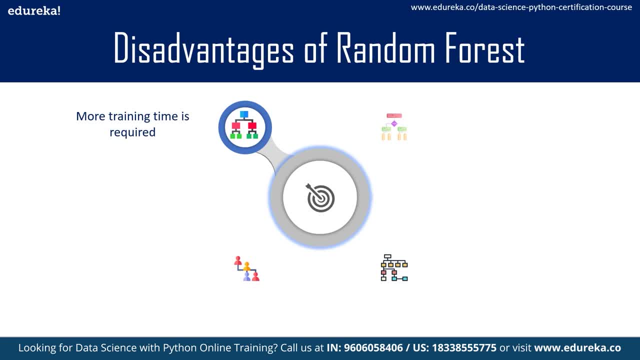 So you would be constructing hundreds and hundreds of decision trees And that requires a lot of training time. And here comes one more disadvantage is that the interpretation becomes really complex when you've got multiple decision trees. So decision tree interpretation is easy because it is an individual decision tree, But when you combine hundreds of decision tree to form a random 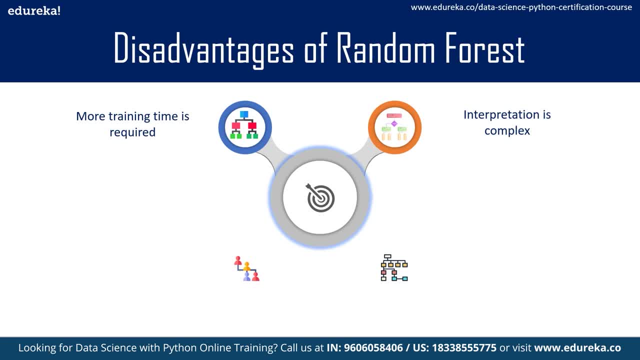 forest. the interpretation is really very difficult to understand and becomes quite complex to apprehend what exactly the model is trying to predict and where the splitting occurs and what features are being selected and so on. And another disadvantage is that it requires more memory, So memory utilization is really heavy in. 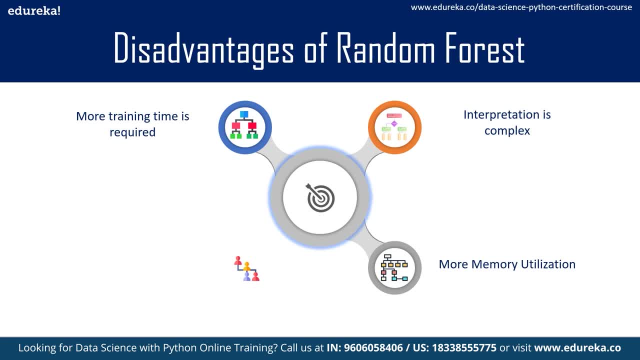 case of random forest, because we are working with multiple decision trees, And another disadvantage is that it is computationally expensive and requires a lot of resources because of the training of multiple decision trees and also storing them. All right, so this was all about. 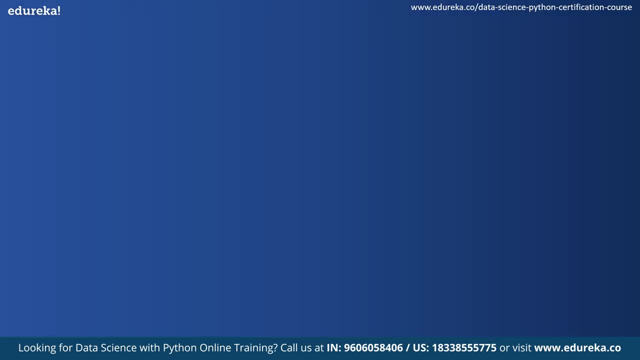 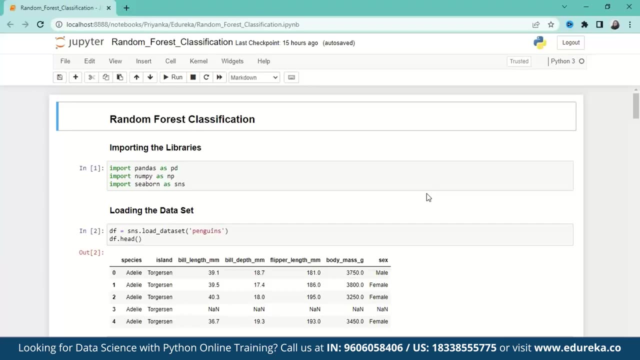 random forest, the theory part of it. So thank you so much for watching this video. I hope you enjoyed it. And now let us just move on to the practical demonstration or a hands-on on random forest. Okay, so, now it's time for a hands-on on random forest, So let us just import a few basic. 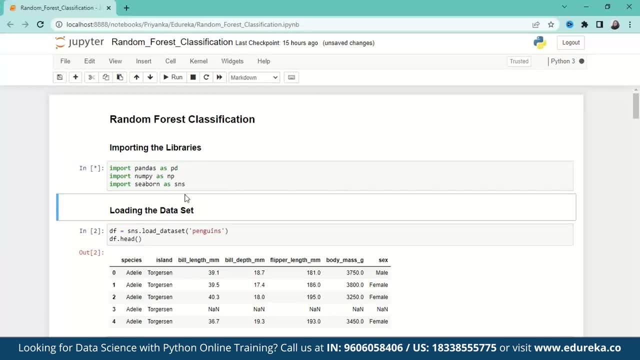 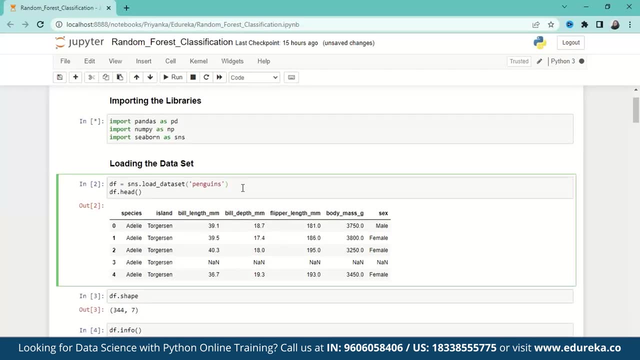 libraries of Python in our Jupyter notebook And we will run this. we will import pandas as spd, numpy as np and seaborn as sns. Now, seaborn is needed here because we want to load a dataset, that is, a penguins dataset, with the help of seaborn, And this has already been. 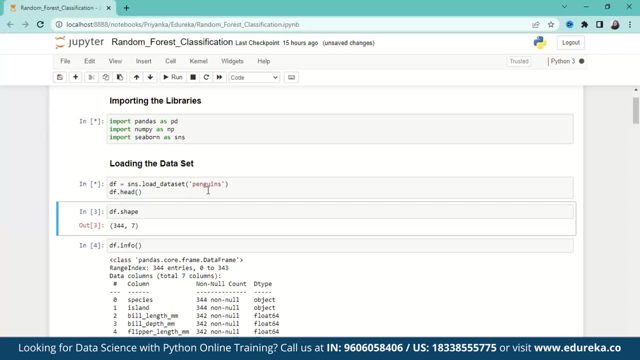 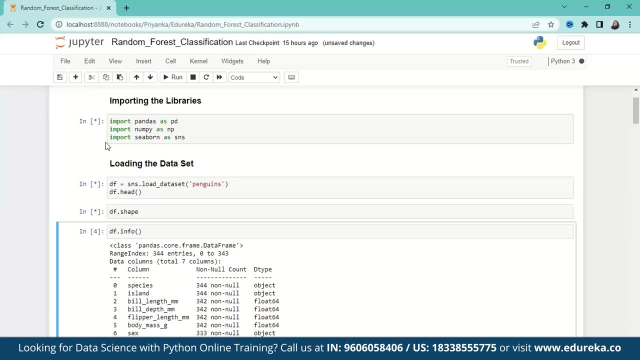 preloaded in seaborn. This is already loaded dataset And seaborn has got multiple datasets, you know, for practice for beginners. So it is a good way to practice for datasets. Now we can see this asterisk sign. that means it is telling us to wait. So let us just let it get. 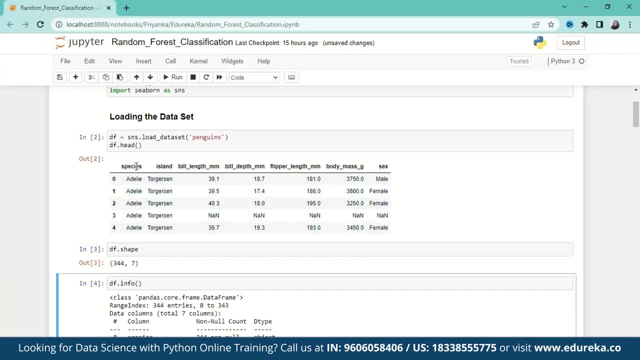 loaded. So we get got our data in an object called DF And we can see the first five entries here, And this data frame is shown in the form of a table, rows and columns, And we see here some species are then build length, build depth, flipper length. 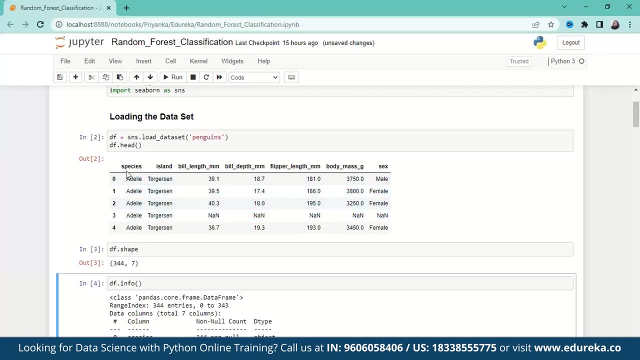 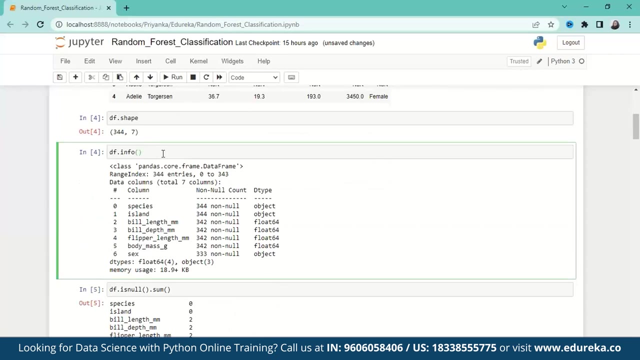 body mass and the sex of the penguin. So our task is to specify or to classify these species of penguins and do their respective correct species right. So we see the shape of our data and we see that it is like 344 rows and seven columns And we will see the info. So we see. 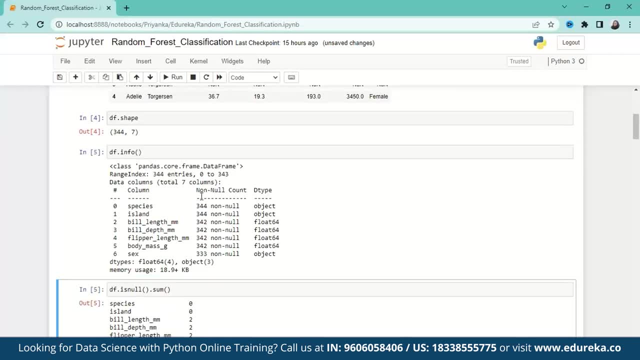 dfinfo And this gives us, along with the non null count, we also get the data type of the values. So we have got species island as the object data type, whereas the build length, build depth, flipper length and body mass are in floating point. or you can say: 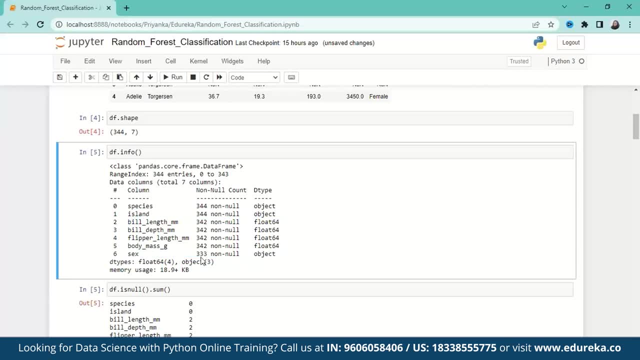 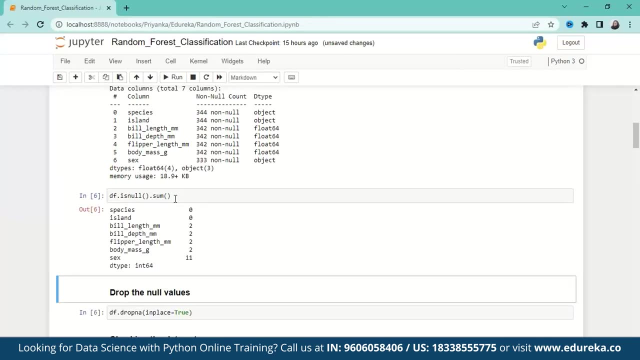 floating data type and the sex is in object data type: right. So now moving on forward to calculating how many null values are there with the help of dfisnullsum. So we get certain like sum around two null values in all these columns. as you can see the features like build length. 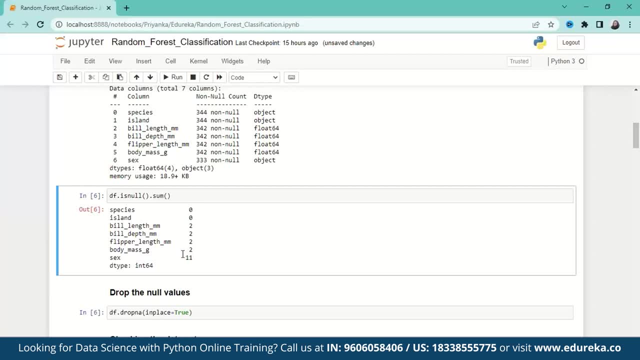 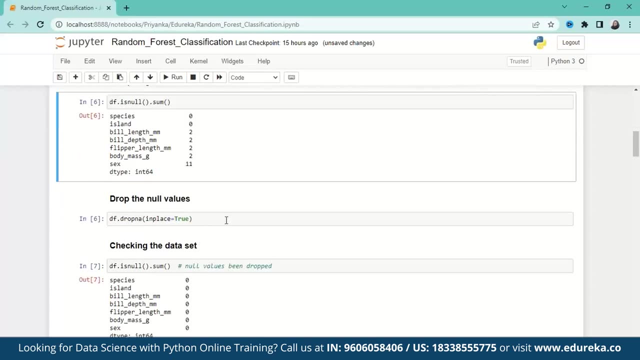 build depth, flipper length and body mass, whereas there are 11 null values in sex feature. right, So do is. since they are very small null values, we can just drop it, or you can also ignore them. So here in this data frame, what I'm doing is I'm just dropping these null values And let us just 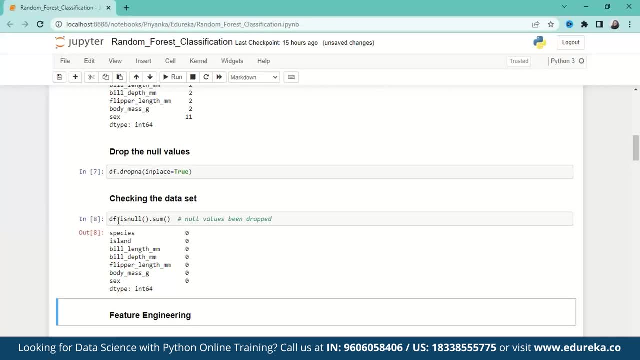 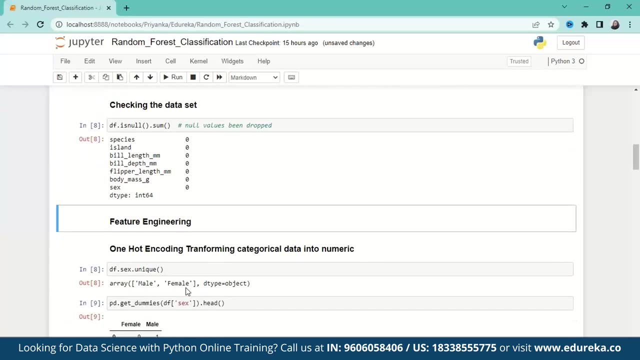 check whether they are being dropped or not with the help of again the same function: dot is null, dot sum. And then we see that, yes, they have been dropped from our data frame. Now let us do some feature engineering with our data. Now we have seen that we have got some object data type in. 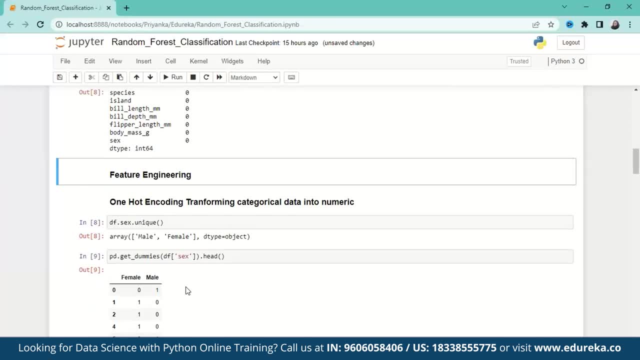 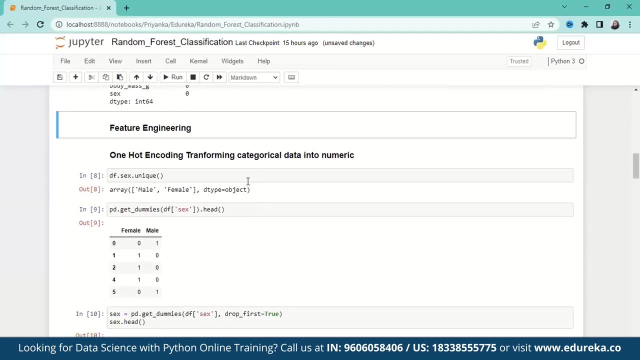 our data frame And before feeding it into algorithm that is random forest, we have to transform the categorical data or the object data type into the numeric. So we are using here one hot encoding to convert the categorical data into numeric. Now there are various ways in Python which we can do that like we're not encoding or 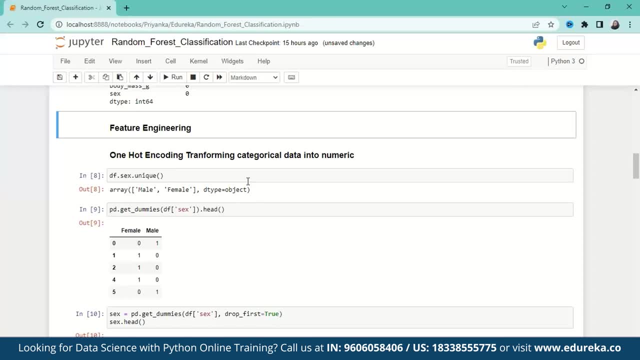 you can also use the mapping function in Python, But here we are using one hot encoding. So let us just do that And we find here. first of all, let us apply it on the sex column, And here we see that we have got two unique values in sex, that is, male and female. 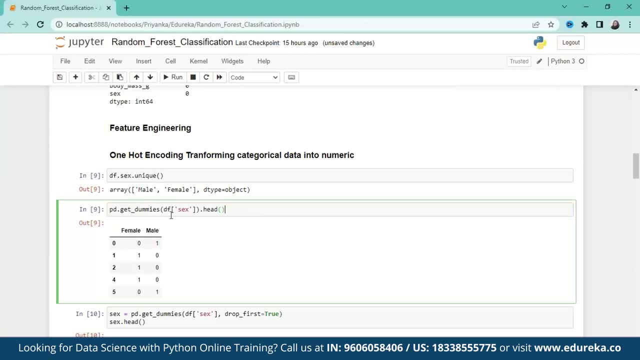 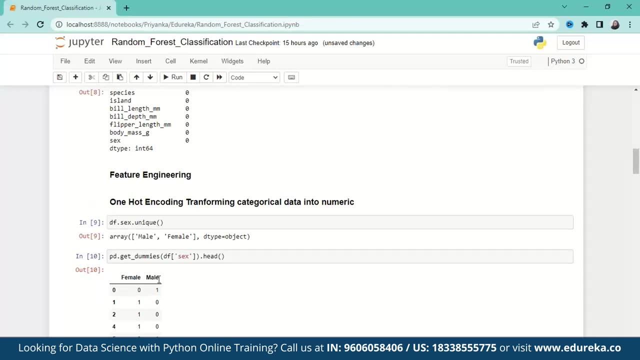 And we use pandas here to get dummies. That is how we will apply this one hot encoding, because this is how get dummies work. So what happens is here is that the new unique values are converted into the respective columns in the data frame. So we see, here we have got two unique values. 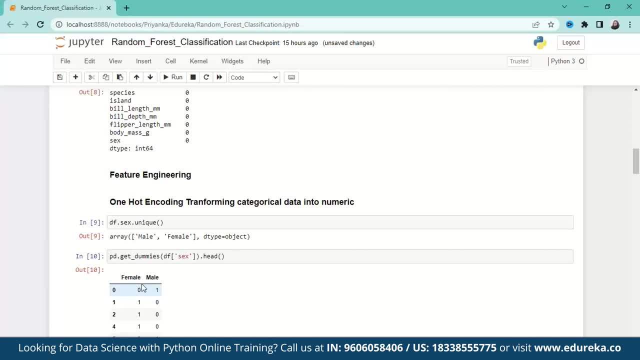 males and females, and they are being converted into the columns. Okay, so one thing to note here is that we also get a problem of dummy trap, because here we see only two unique values. Now suppose if I had six or seven unique values and I do this one hot encoding, I would have lots of features in my data frame. 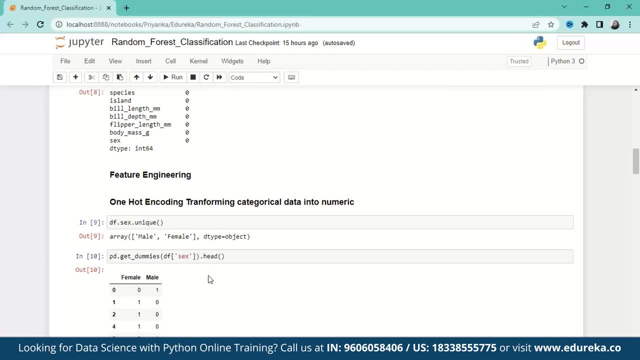 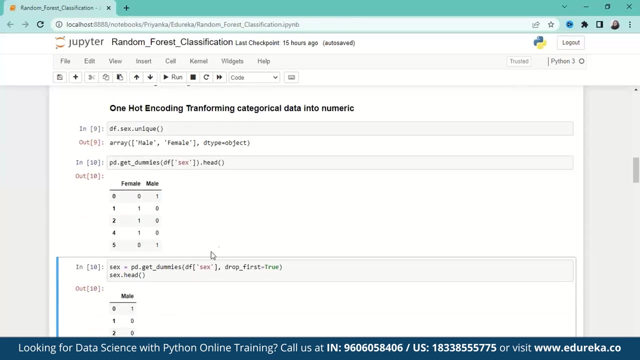 and that would lead to several complexities. So what I do is to keep things simple. I can use one hot encoding when my data frame or my unique counts are low, when my unique values are less. So since I had just two or three, I can use it, So I'm using here. So what I do is again now one row. 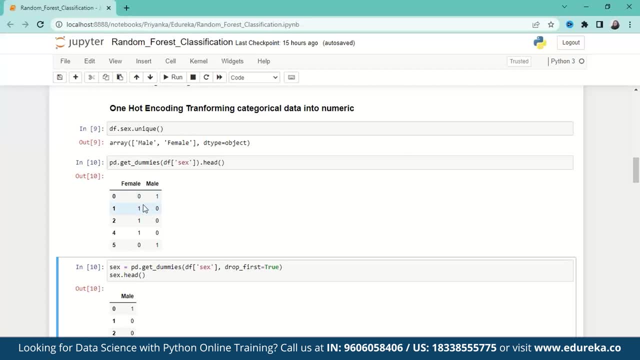 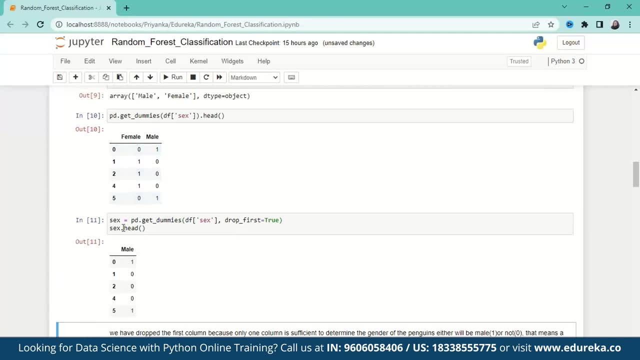 one column, as we can see here that it is redundant giving me extra information, So I will just drop it. So I drop this first column and what I get in this data frame is only male. So let us just infer whether I can also infer females from this or not. So if the value is one, that means 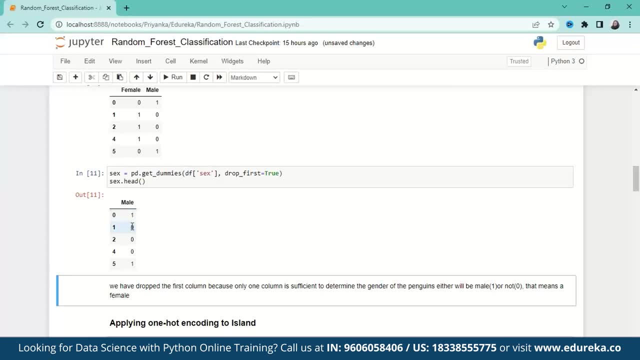 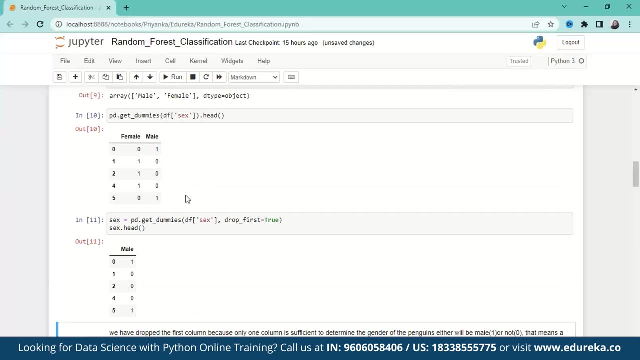 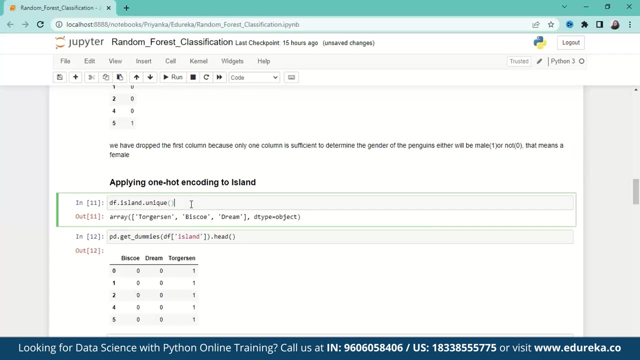 the penguin is a male, and if the value is zero, that means the penguin is a female. Okay, so only one column is needed for this data frame. So I just kept one and drop the other one. Okay, Now apply again one hot encoding to the island feature. So in island, if we check the 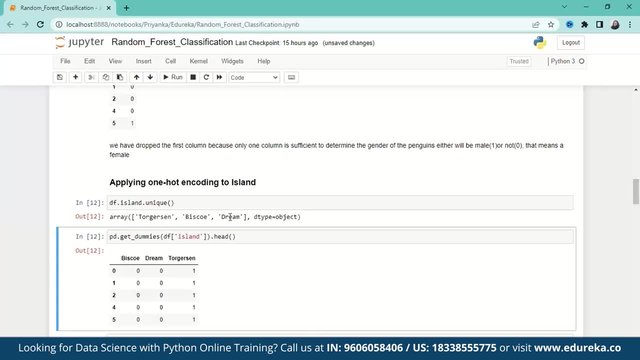 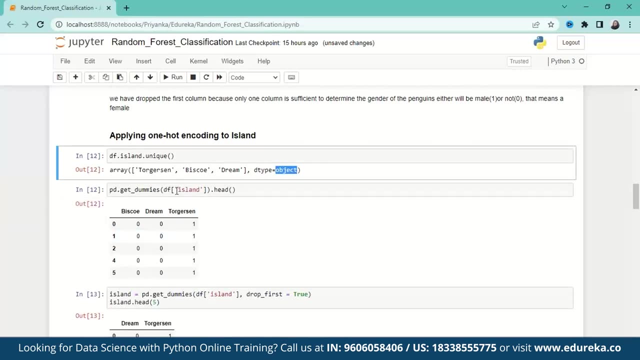 unique values. we've got three unique values here: Togerson, Biscoe and Dream Island- and the object is the data type, right. So again we will use pandas PD dot, get dummies. and we will use apply it on the feature Island and let's get the head of it. So we get here again. the unique values were: 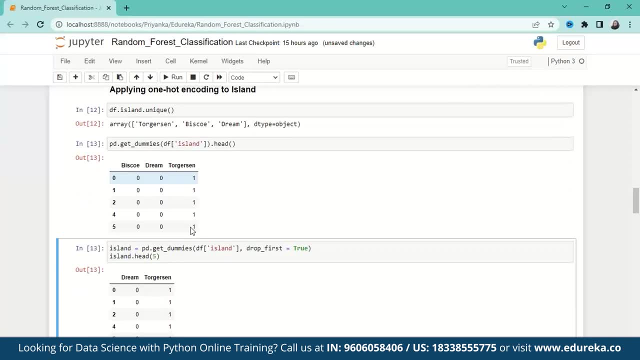 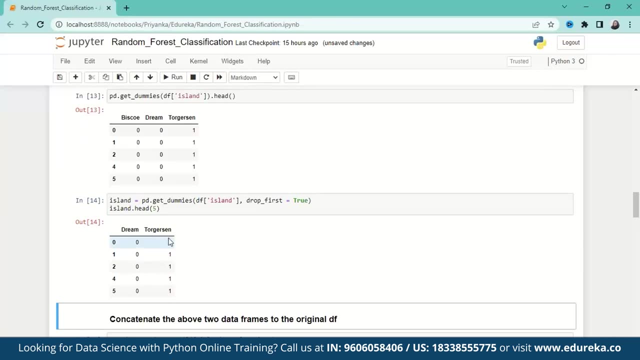 converted into columns and we get here respected three columns, and then again we will just drop the first column to get the remaining two columns. So here also we can infer that if the island is Togerson, if it is one, then it is not dream, neither Biscoe, right? So this is how you can. 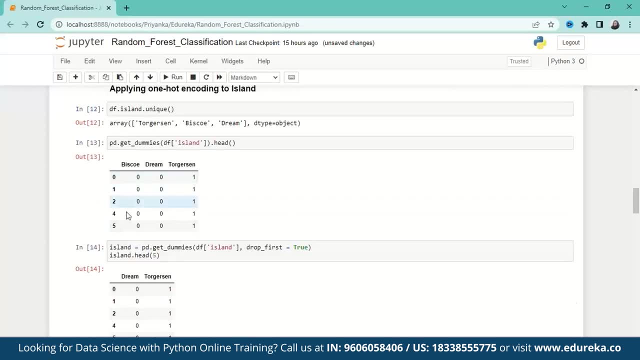 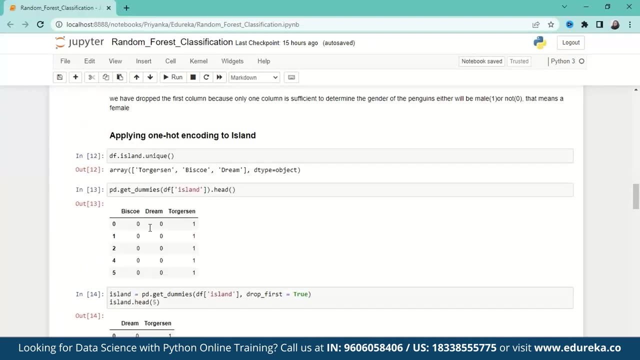 read it from the data frame and understand that. now remember this thing: that these two Island and here sex. These are two independent data frames. These are not yet included in the main data frame. So what we will do now is we will concatenate the above two data frames into the 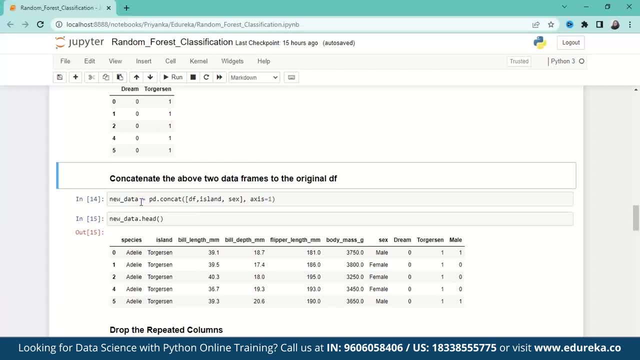 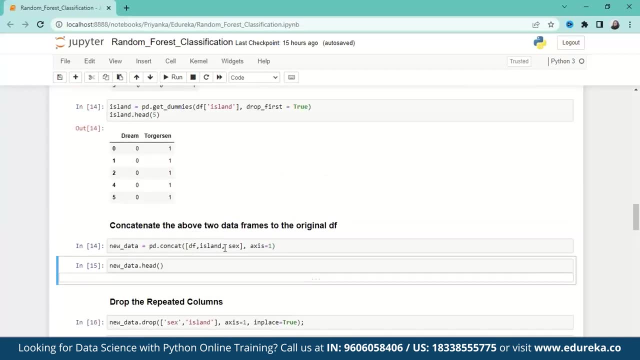 original data frame. So what we do? we again create a new data frame, that is new data, and let us just concat with the help of PD dot concat function and we will concatenate what Df, Island and sex and X is 1, that means in the column. Okay, so when we will run this? 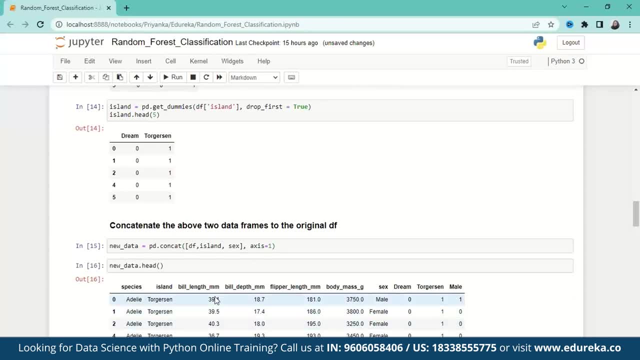 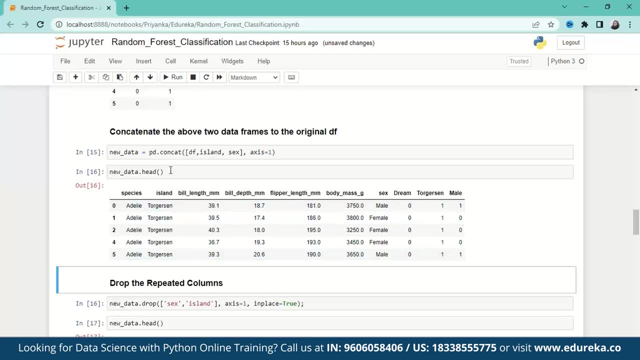 let's see the head of it. So everything gets concatenated in a single data frame, which is good. further feeding this data into, or splitting the data into, test and train data. So now we have this new data frame and we've got some repeated columns here, which needs to. 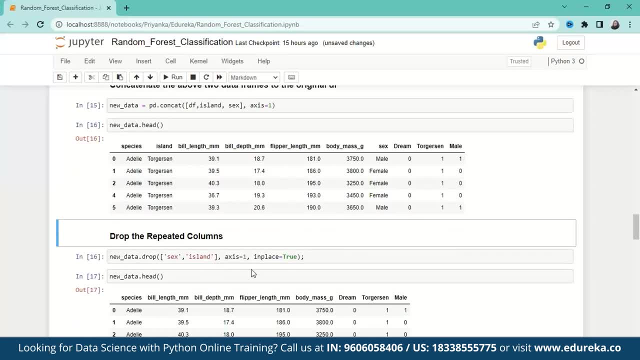 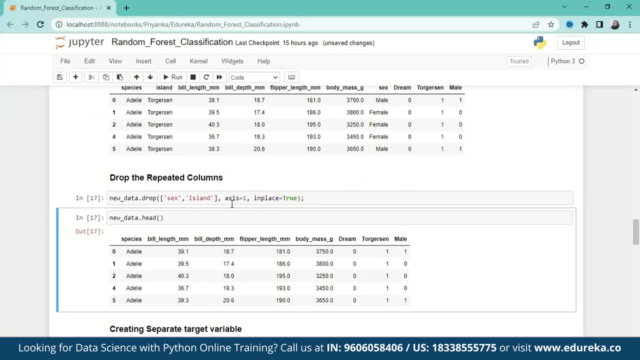 be deleted. So what we do is we will delete sex and Island here, which are just repeating, because we've got here mail and we have also got here dream and Torgerson. So we do not require this Island column, neither the sex. So we just drop it with the help of new data drop and the column names: X is 1 in place equals to true. 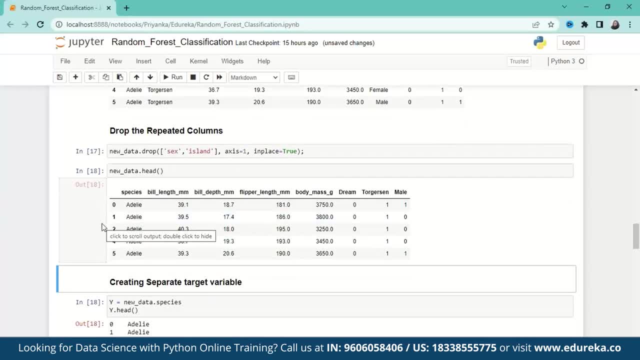 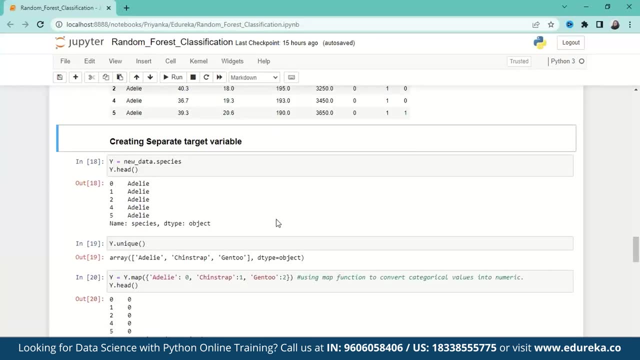 right, and let's see the head of this data frame. head of the data frame gives me five unique values. right and now it is time to create a separate target variable, and what we'll do is we will store in a variable called by only species. So what we do is, from this new data dot species, We will just 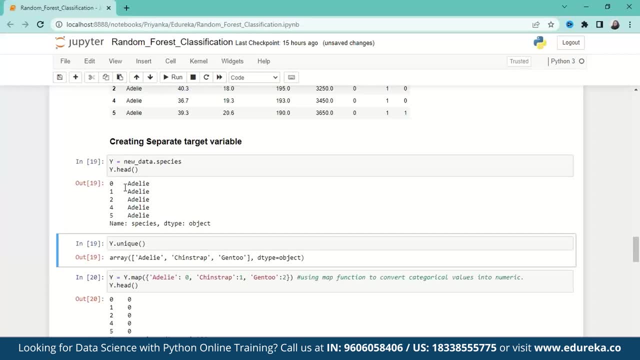 store the species in this pie and we see this by a dot head. That is the first five species and we got the values here. That means another target variable is being created now, So and you can also see the y dot unique values as a deletion strap and again to so now we see here three unique 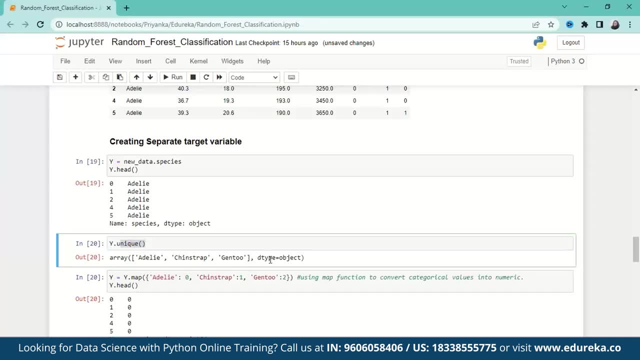 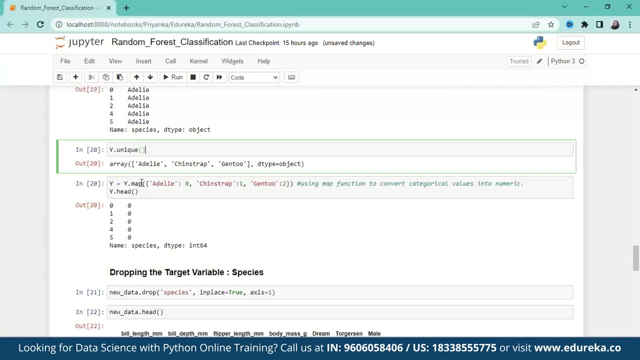 values of the penguin, that is, chin strap, Italy, and again to, and the data type is object here, So again, we need to convert this object into the numeric data type. So now what we are doing is we are using the map function in python. 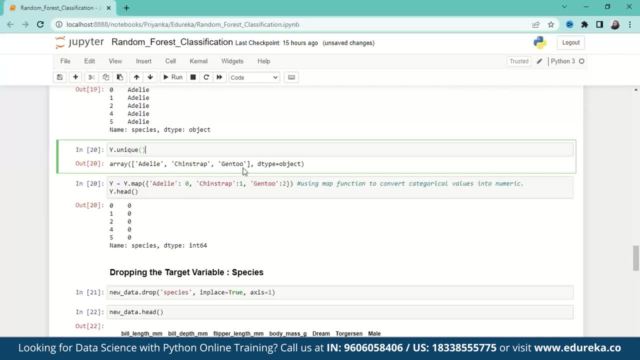 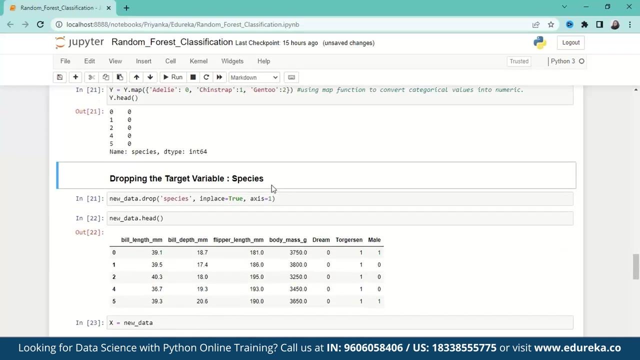 And what we do is we map Italy to zero, chin strap to one and can do to two. So this is how we see, then all the values have been mapped to numeric. This is another way to convert a categorical value into a numeric value in python. Now what we do is let us just drop the target value species. 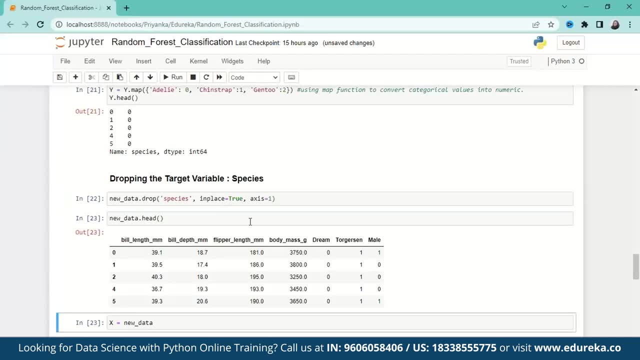 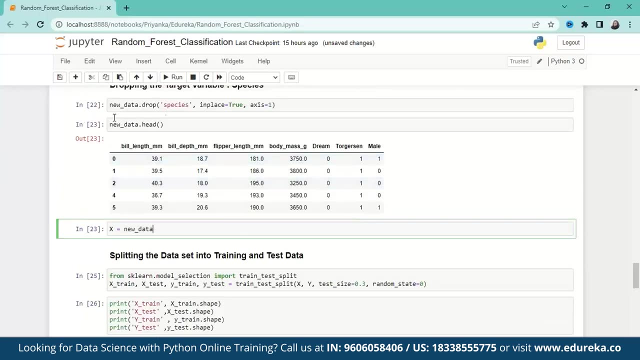 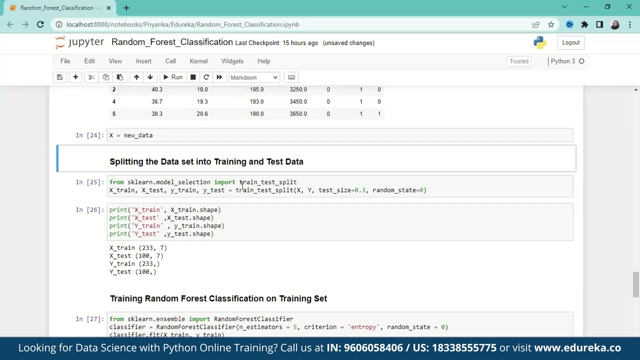 from a main data frame, So we just drop it. and let's see a new data frame. So we see that we don't have any target species here, right, Okay? So in X let's store this new data And perform the splitting of the data. So what we do is: from sklearnmodel selection. 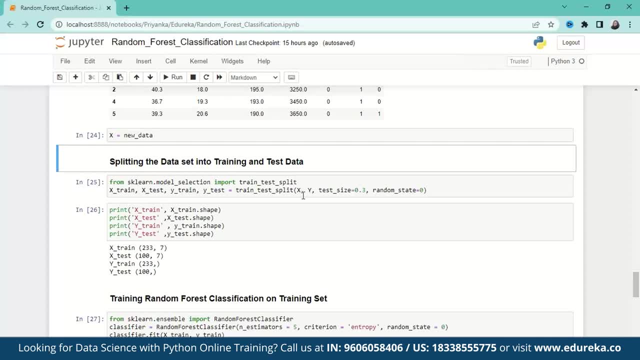 we will import our train test split and we will split our training data into 70% and 30%, or test data becomes 30% and training data is some 70% and this random state is zero, which means that I'm not fixing any random state, and this is also used for the code reproducibility. Now suppose if 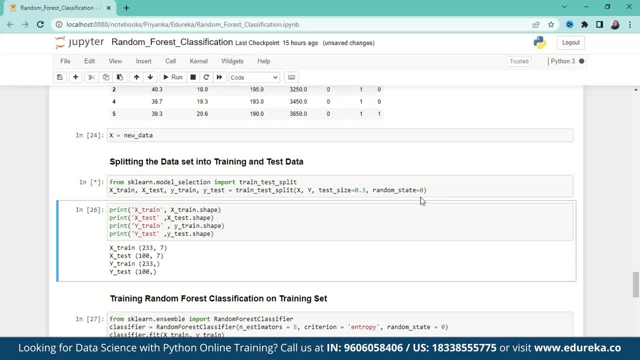 I again run this code. I will get the same result. It will not change. You can set this random state to any of the random number as per your choice, and the result would differ. Okay, so now let us print the shape of X train by train, X test and by test. So we see here that it has been split. 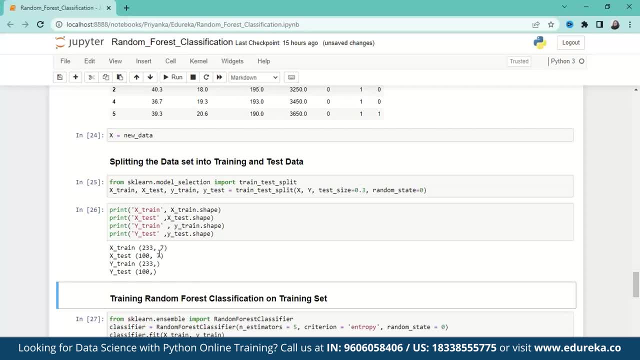 it into 70 and 30% and we get X train as 233 values here and seven features, and X test has 100 values and seven features. Similarly, by train you can see 233 values and Y test has 100 values. That means the species. Okay, so that has been perfectly split it. 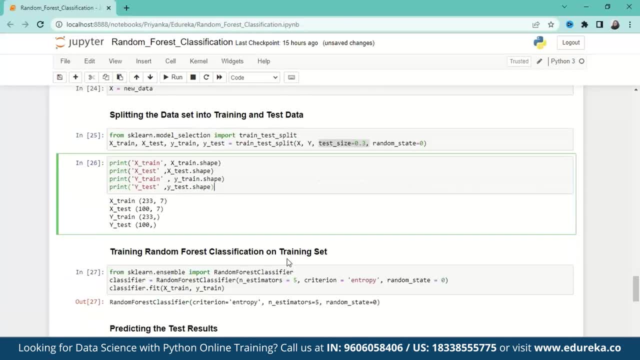 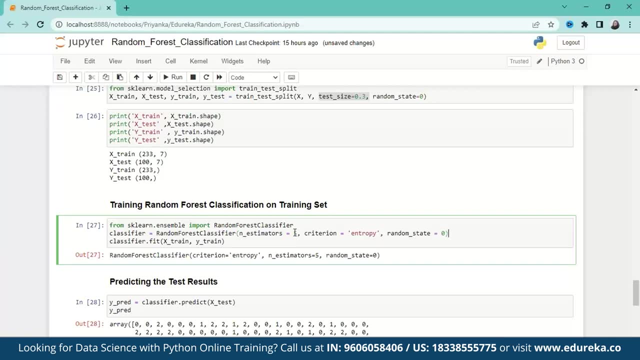 into 70 and 30%. Now what we do is we will train the random forest classifier on the training set. How do we do it? we will import the random forest classifier from sklearnensemble- So we've already dealt with what is ensemble- And then in classifier we will store this random forest and this. 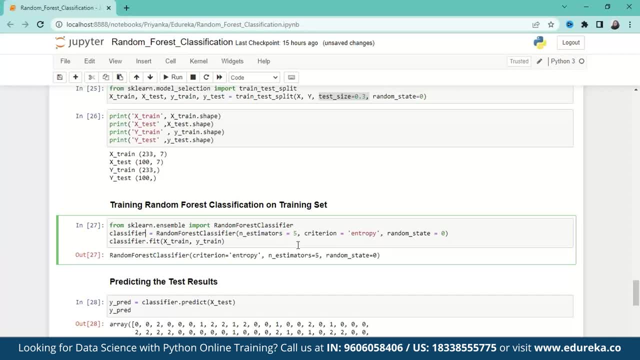 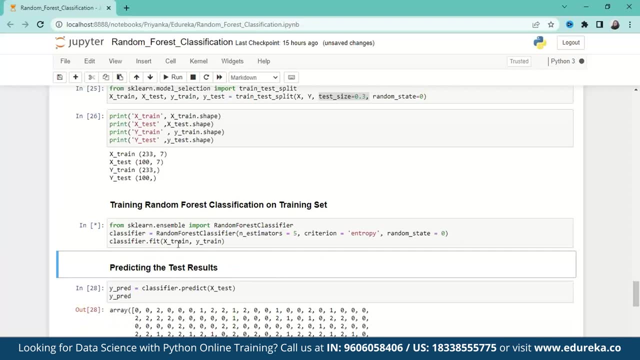 n estimator is nothing but decision trees. So we are creating some five decision trees here And the criteria is entropy And again random state is set to zero. So let's see, And then we will fit this X train, And by train. so this has been fitted and the criteria is entropy here. Alright, so now let's. 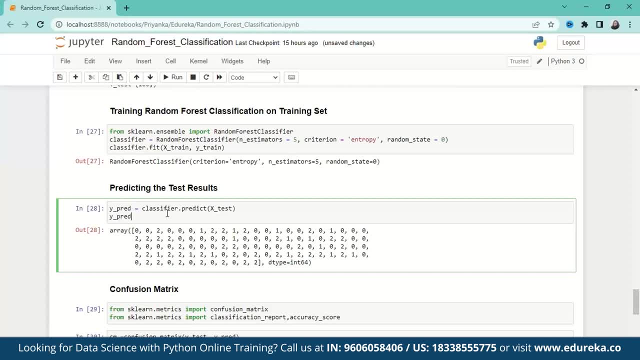 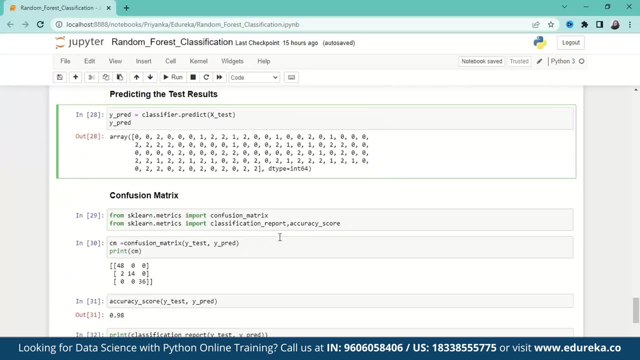 make some predictions And let's create a variable called vibe predict And we will just predict it on X test And we've also printed this vibe prediction. And now let's bring the confusion: matrix to check the accuracy of random forest algorithm. And what we do is from matrices. 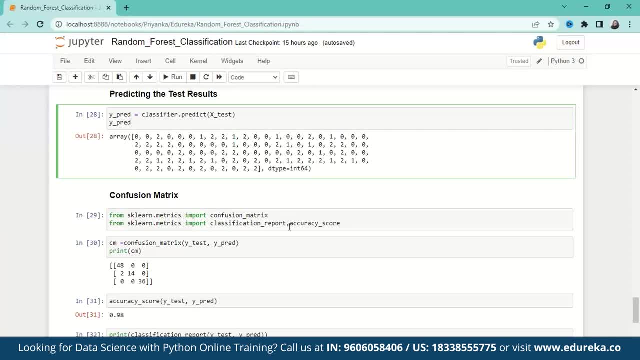 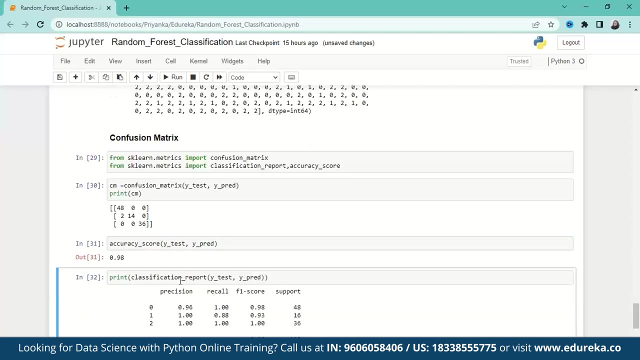 sklearn matrices: we will import classification report and confusion matrix and also the accuracy score. So we will just import them. and then CM variables: we will print the confusion matrix of Y test and Y predictions. So we will print it and we see here the accuracy score also, which is 98%. So our random forest classifier is giving us. 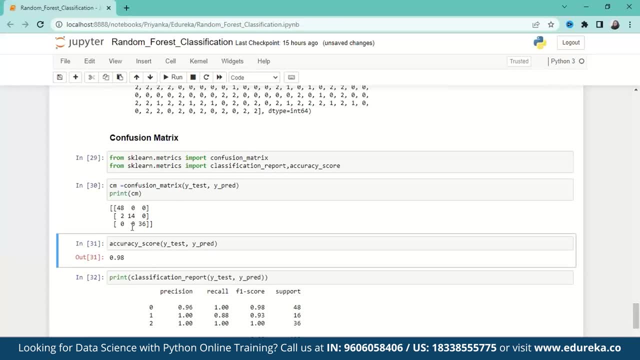 a very good accuracy of 98% And you can see a confusion matrix that only two cases have been misclassified. Rest, all the cases have been correctly classified by random forest classifier. Okay, so now let's move on to printing the classification report of Y test and Y predict. 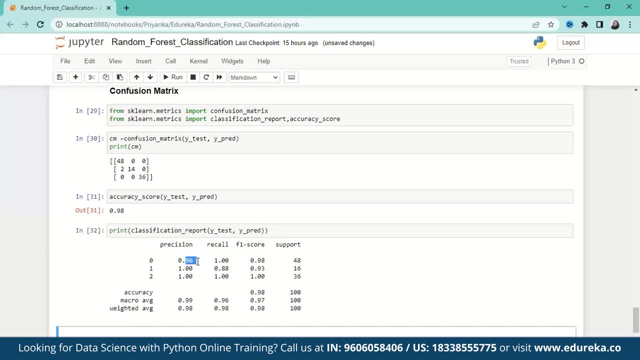 Let's see. And we get the precision as 96%. That means the two predictions by the algorithm is 96%. The recall, or the true prediction rate, is 100%, which is very nice, And Evan score is also good, which is 98%. So this is giving us a good result. But what if? if we change the criteria from entropy?